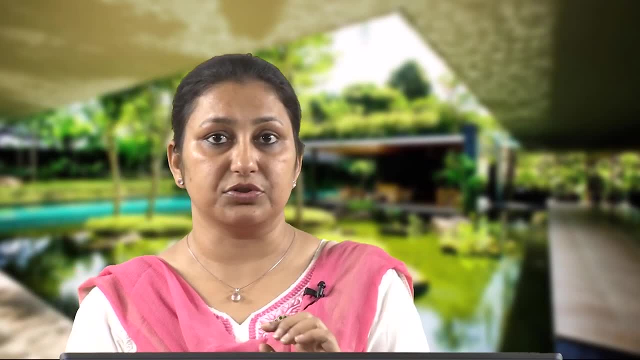 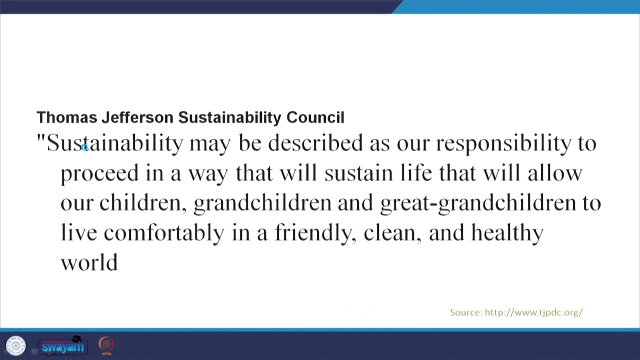 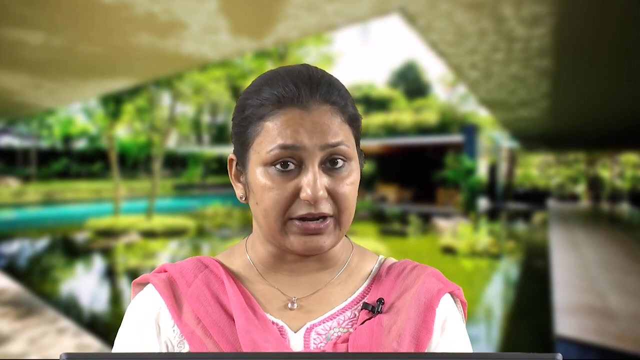 let us look at the key words in each of this definition. First is: we have to proceed in a way that will sustain life. So we have to sustain the life in a way that is comfortable, friendly, clean and healthy, which implies that the environment 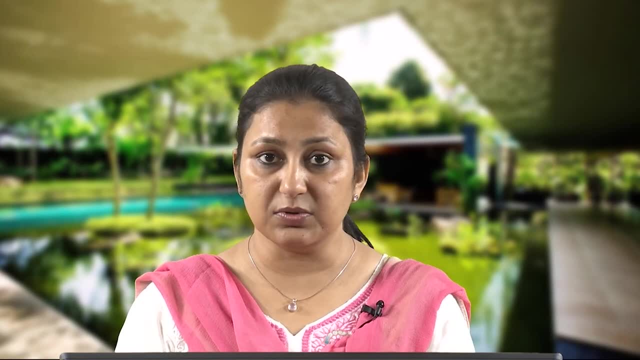 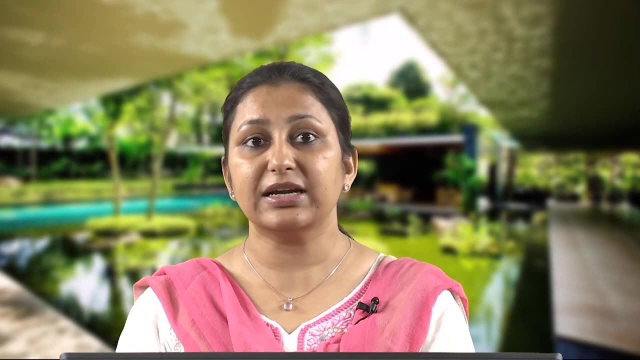 is good for our future generations. they are comfortable, so they have enough resources to sustain themselves, flourish and they have a friendly environment that obviously they are going to raise their kids mentally. They are going to make them happy. then they are confident in themselves and enjoy the playground which is 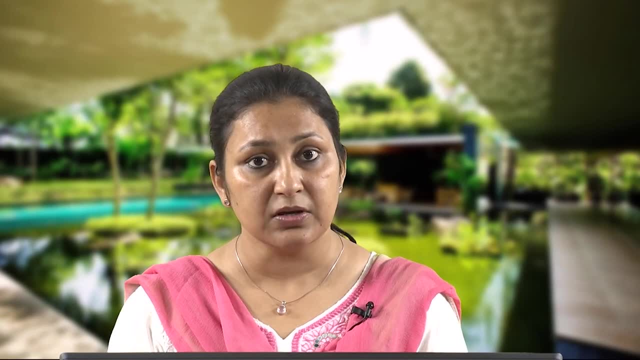 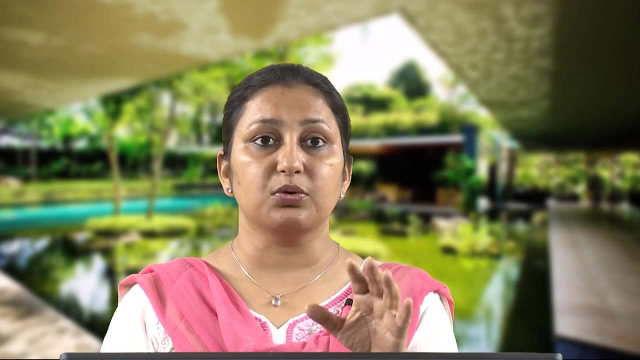 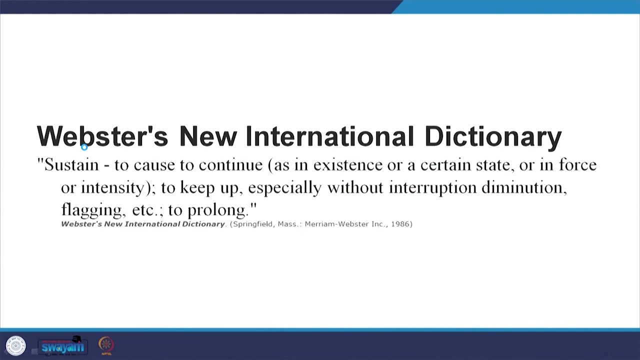 which is socially and culturally thriving. So this is what we are meaning when we are looking at this definition. Let us look at another definition. So if we look at the Webster's International Dictionary, the word sustain literally means to cause or to continue. 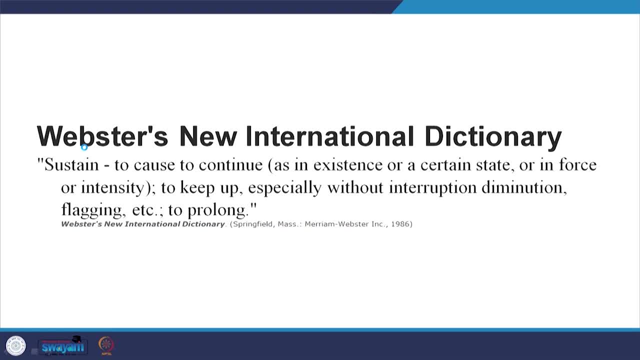 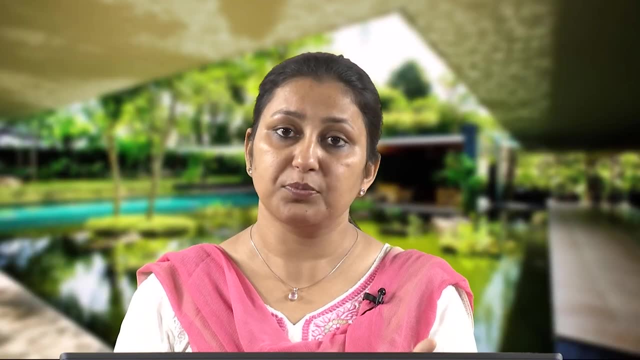 as an existence or a certain state, or in force or intensity, to keep up, specially without interruption, diminution, flagging, etcetera, or it is to prolong. So, in whatever state we are today or in any point, at any point of time, sustain implies to continue in the same state. 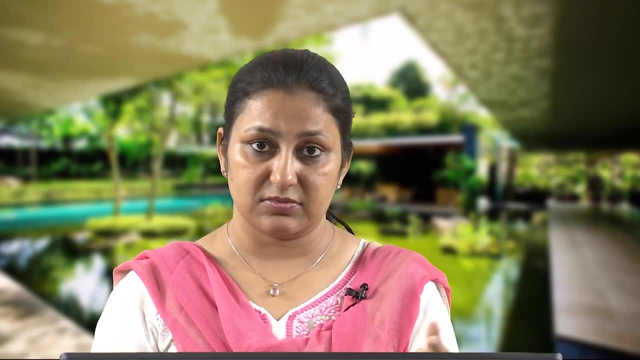 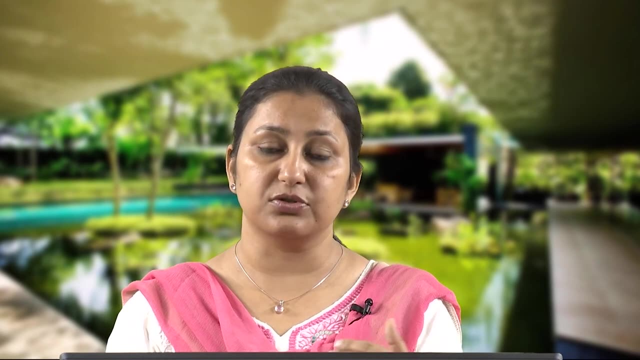 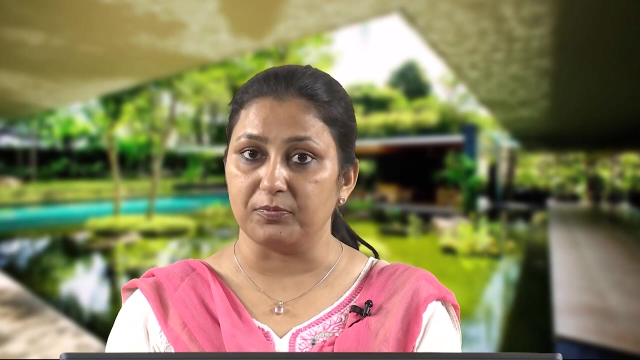 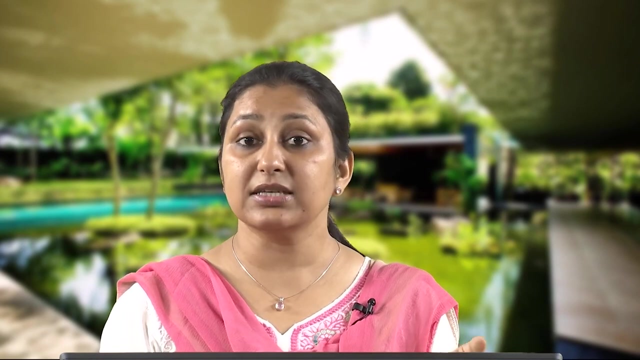 Now, if we look at some time back, say 2 centuries back, at the beginning of industrial revolution was the environment, the overall environment, which includes the socio-cultural context as well. Was it the same at that time as it is now? No, of course it has changed. it has evolved, emerged. 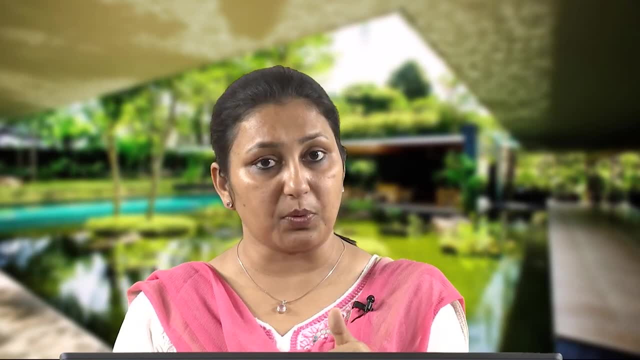 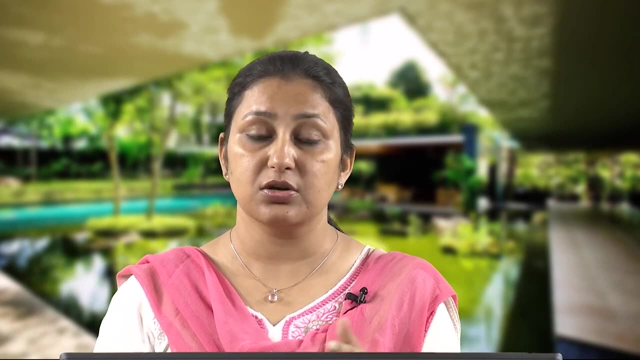 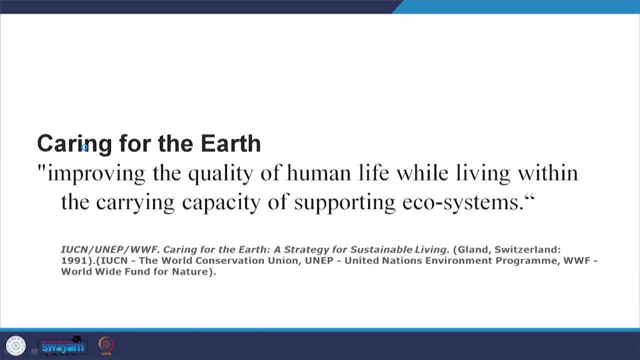 but will we be able to provide the same environment as we have today to our children, to our future generations? Probably not, or maybe yes. So sustain is essentially to continue in the same state. Another definition says improving the quality of human life while living within the 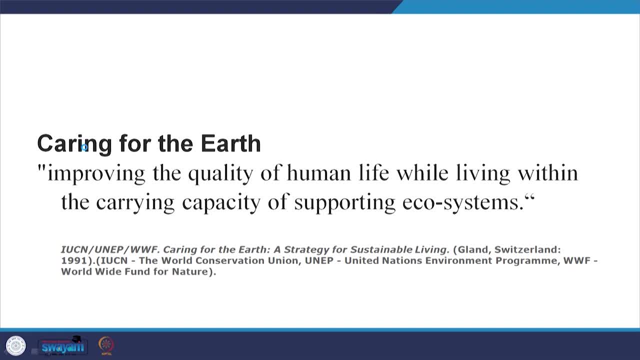 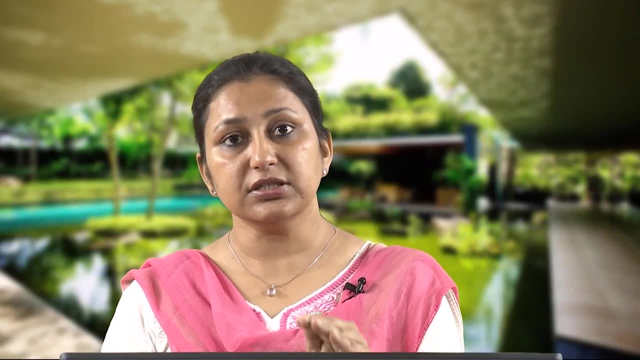 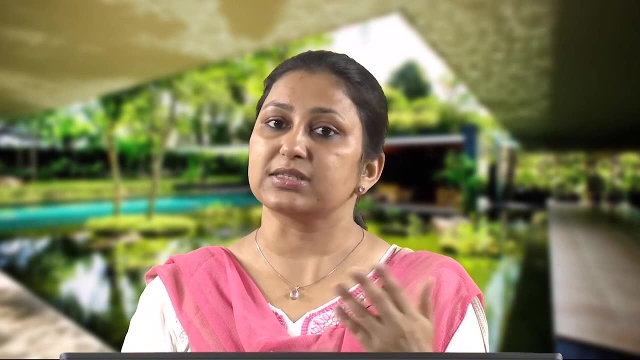 carrying capacity of supporting ecosystems. It is, in a sense, the way of achieving sustainability. So if we continue to live within the carrying capacity of supporting ecosystems, we will be able to sustain ourselves. So it is the process. we have to consume only what is available. 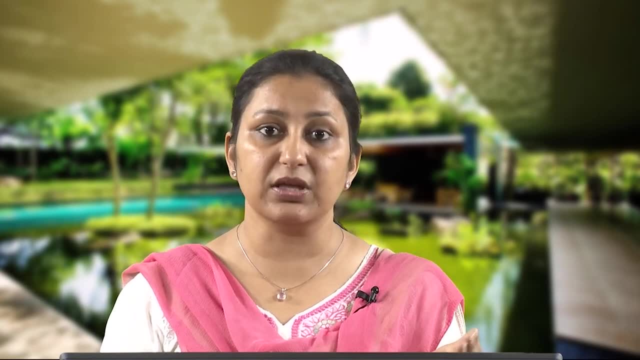 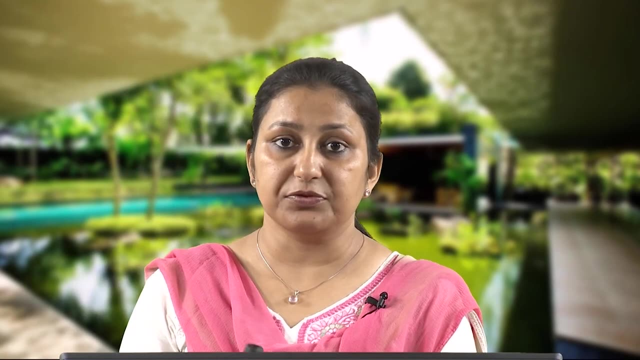 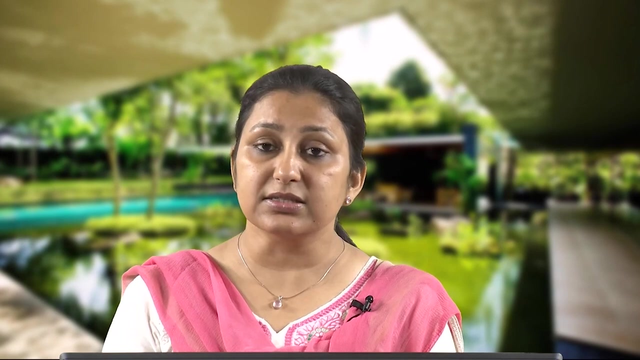 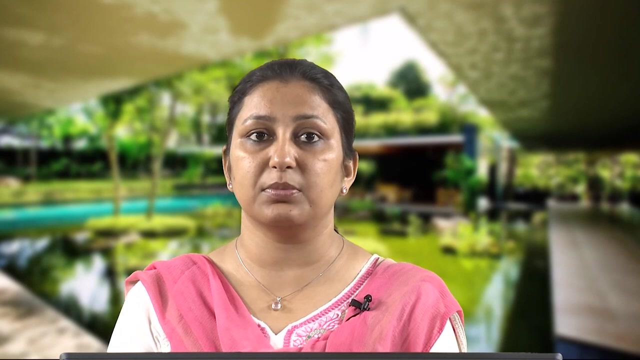 to us say per capita basis, from the surrounding ecosystem. One of the most commonly accepted definition of sustainable development came from the report our common future and it says sustainable development is the development that meets the needs of the present without compromising the ability of future generations to meet their own needs. So it says we are not going. 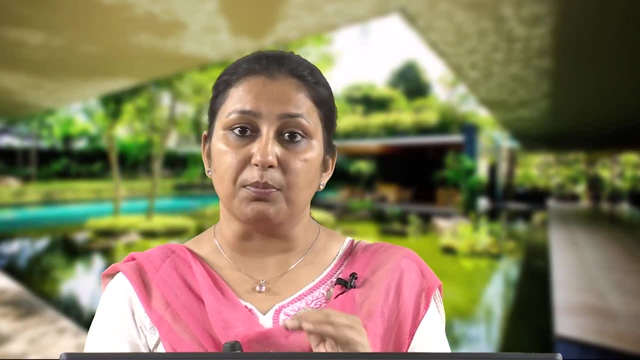 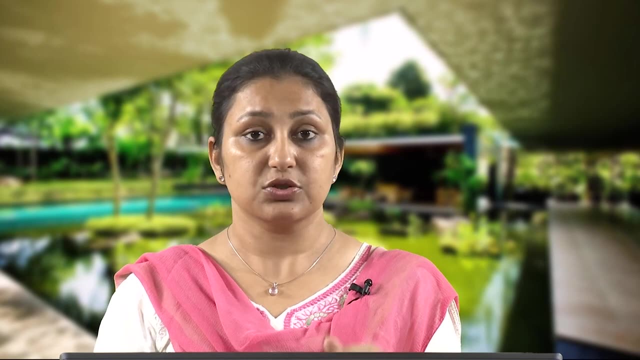 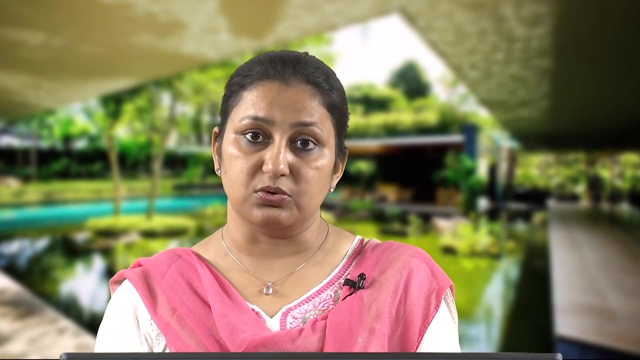 to compromise our own needs of present, but we are also not compromising on the ability of future generations to meet their own needs. So, as we saw yesterday in the previous lecture, the needs can be controlled. We have to frame our needs in such a manner that we are able to. 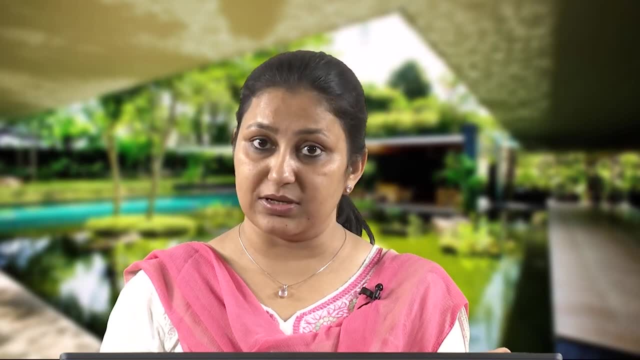 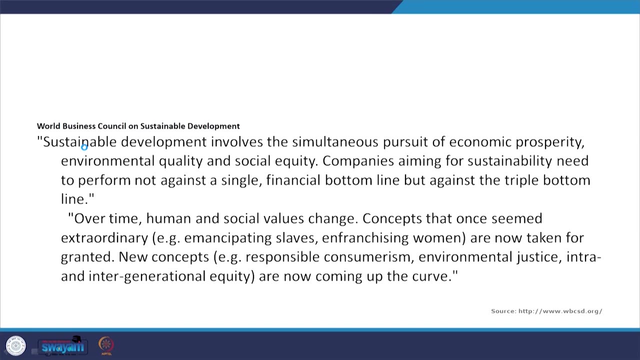 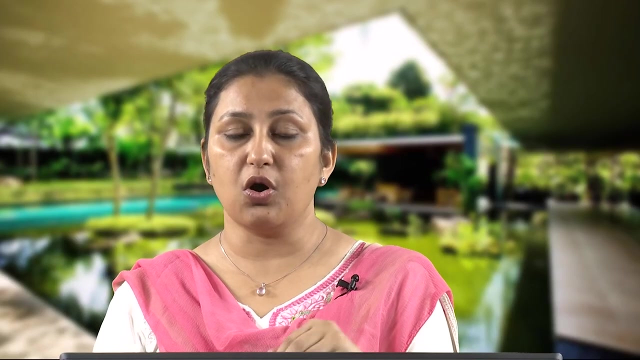 fulfill them today and tomorrow as well, for our future generations. If we look at the world, we have seen the development of the future. We have seen the development of the world business council on sustainable development and how it defines sustainable development. We see that gradually, the focus on economic prosperity, social equity, social justice. 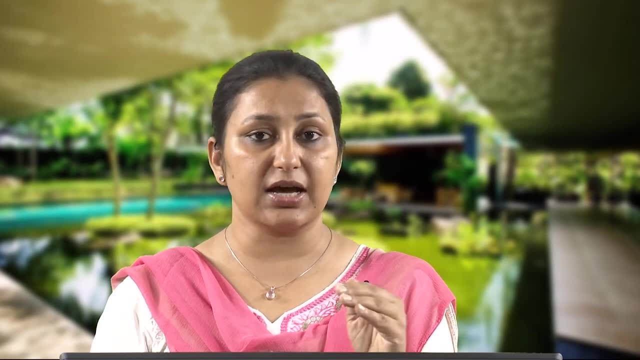 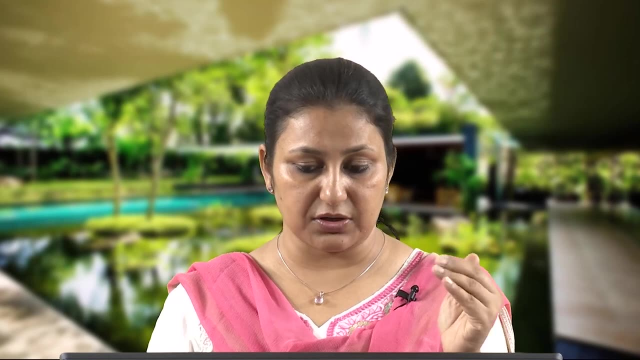 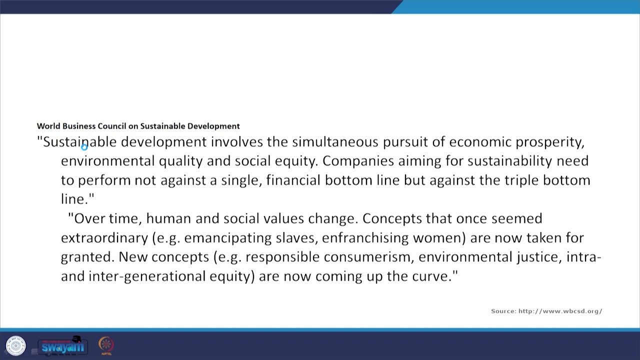 finds a little more emphasis mentioned as compared to the environmental definition, and that is what gets reflected through the definition. if you read: Sustainable development involves the sustainability of the environment. Sustainability of the environment involves the simultaneous pursuit of economic prosperity, environmental quality and social equity. 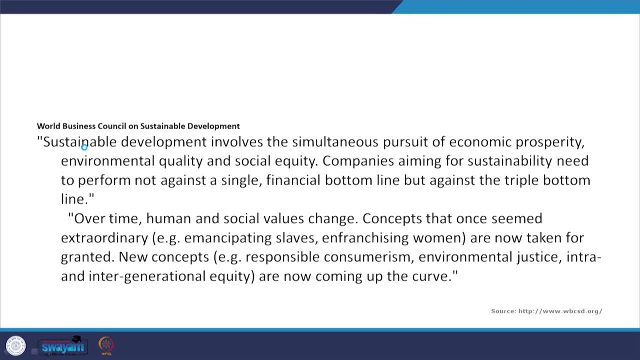 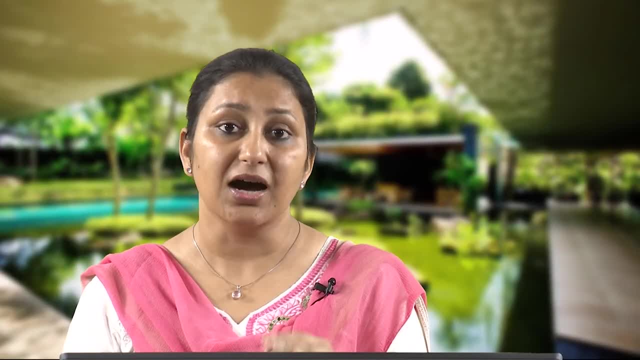 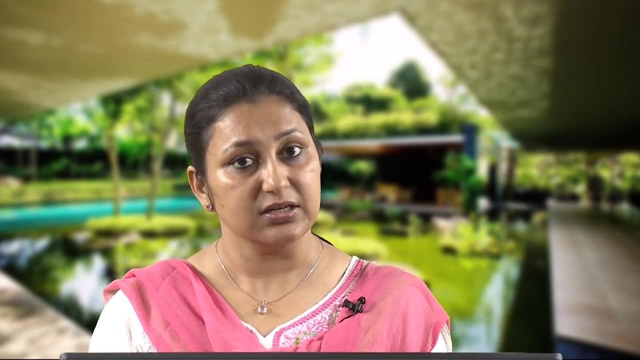 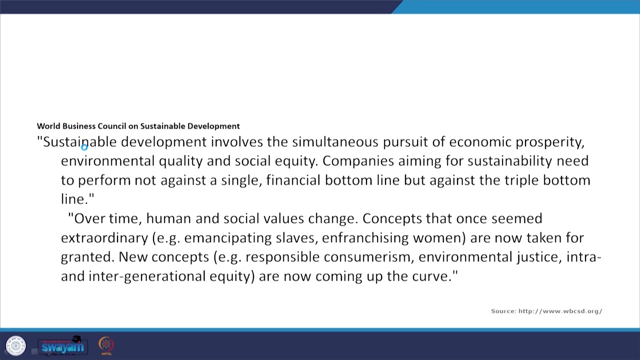 And it says that companies should aim to perform not against a single financial bottom line, which majority of the profit making companies are focused with, but against the triple bottom line which is of environment, social and economic. So some of the concepts, extraordinary concepts in those times, for example, emancipating slavery or enfranchising, 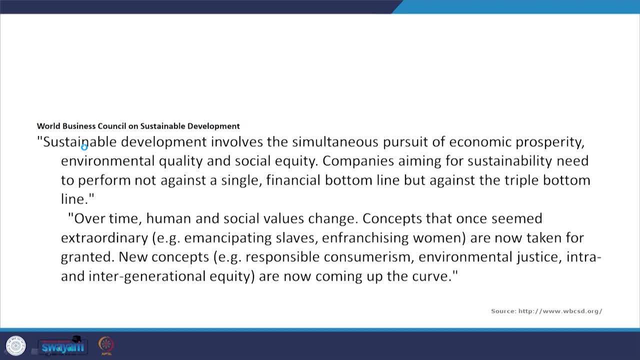 women are now in today's times, they are taken for granted. At one point of time they were like big issues. So similarly the new concepts of responsible consumerism, environmental justice, intra and intergenerational equity. they are now being discussed as big issues. However, in the 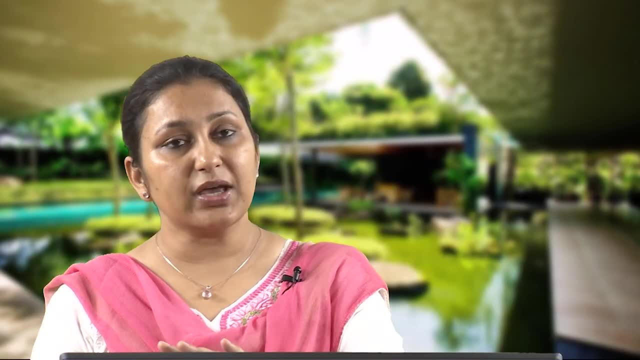 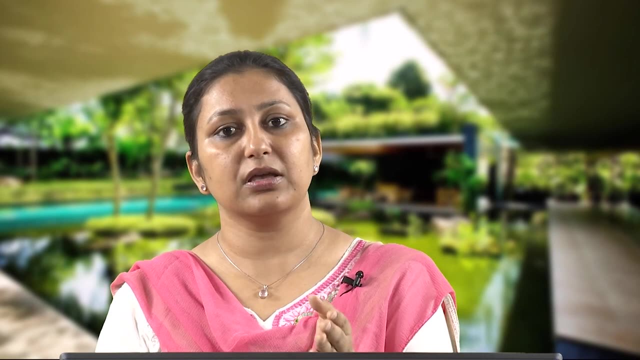 time to come they will change and the consumerism will change And in the time to come they will change. Now, once we have looked at couple of these definitions, we see that some of the points, issues, they keep coming repeatedly in all these definitions, while the focus may vary. 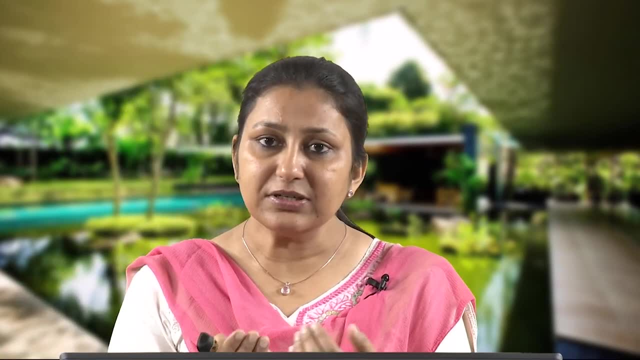 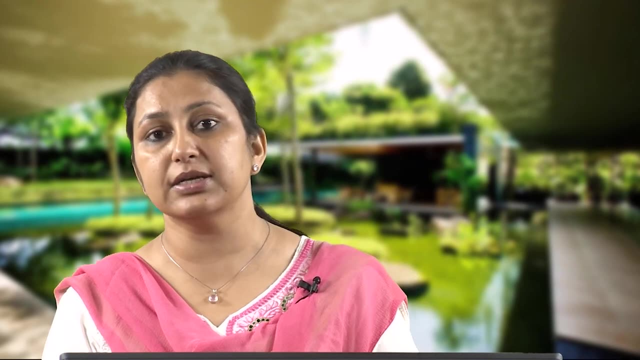 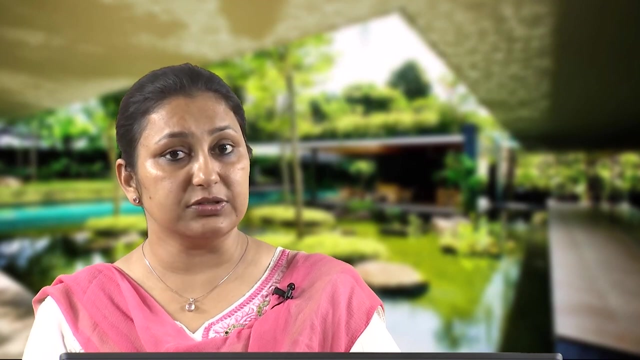 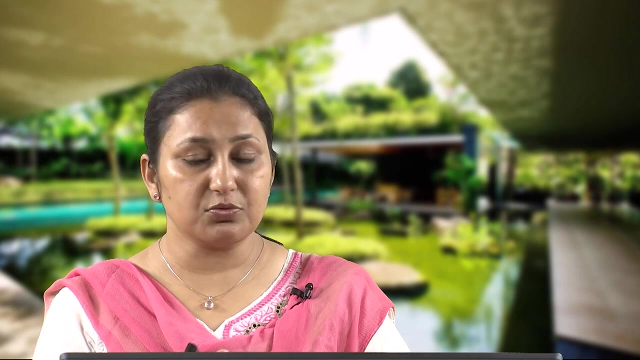 a little bit. So there are different definitions or understandings of sustainability depending upon the point of view, the perspective of who is defining the definition of sustainability. So there is a need to develop scientific models of how to understand sustainability. They could be different types of models, they could be different ways of understanding. 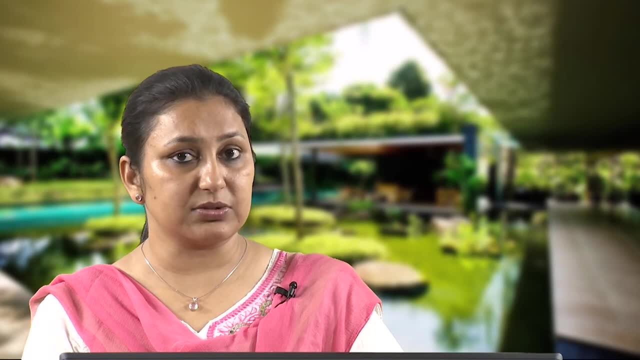 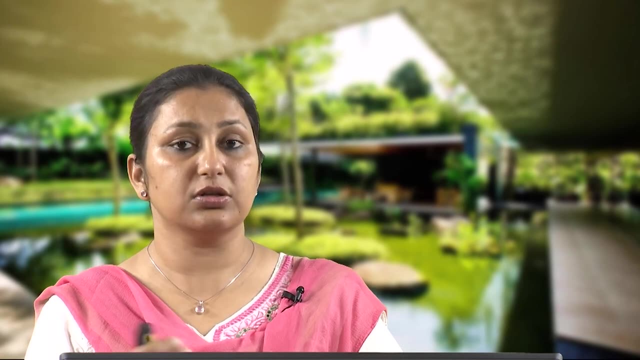 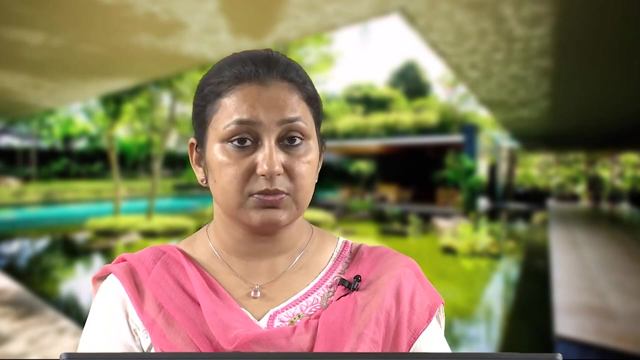 sustainability. But the essential characteristics of any scientific model has to be seen while defining or coming up with a new model of sustainability. We will see couple of these scientific models of defining sustainability In the slides ahead, but the essential characteristics of scientific models must stay. 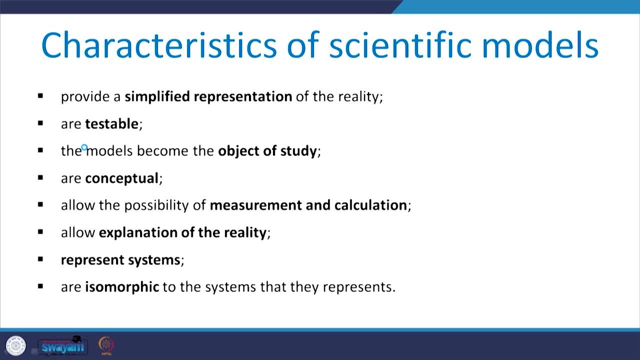 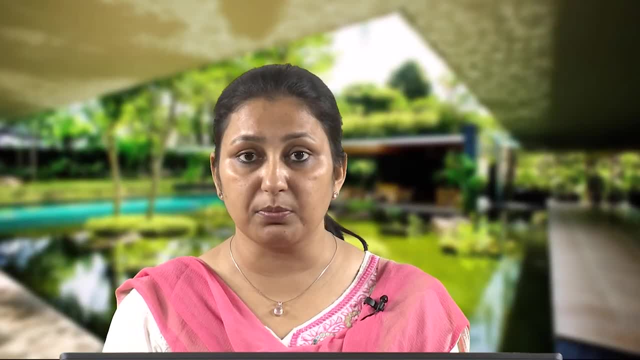 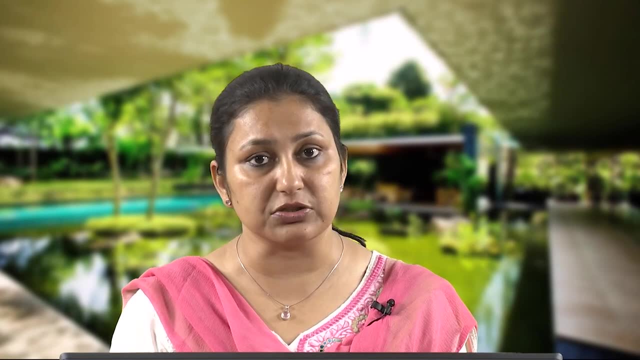 The first and foremost is it has to be a simplified representation of the reality. it has to be very simply conveyed. We cannot make a model which is very complex difficult to understand. It should be testable. we should be able to test the model on different situations, different conditions. It has to itself become the object. 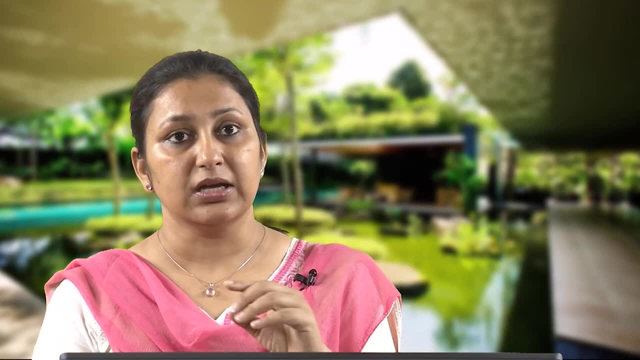 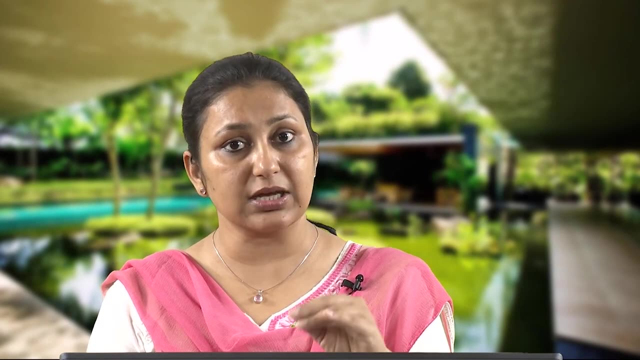 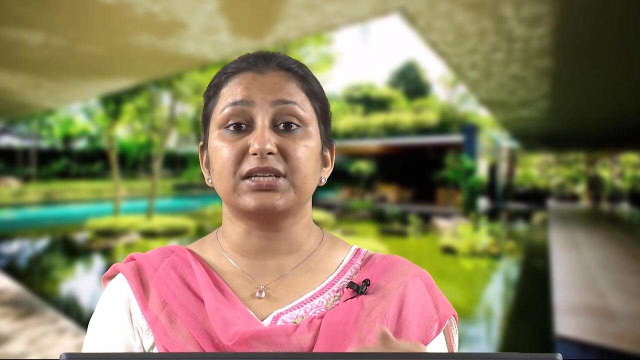 of study which we will see how it gradually becomes. It is usually a conceptual model which we apply to a given circumstance, given context and test it, And it allows the possibility of measurement and circulation. So it has to be tangible, we have to be able to measure it. 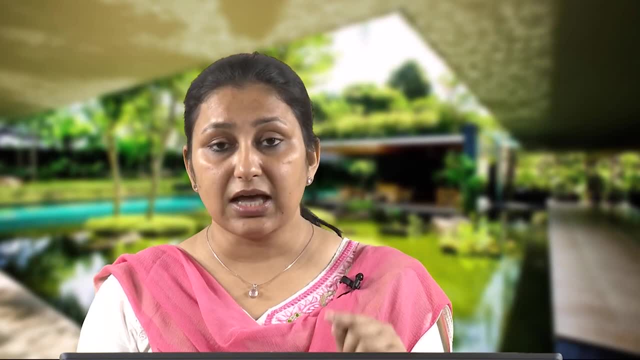 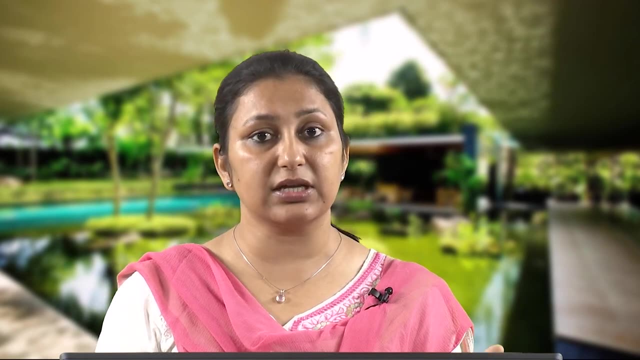 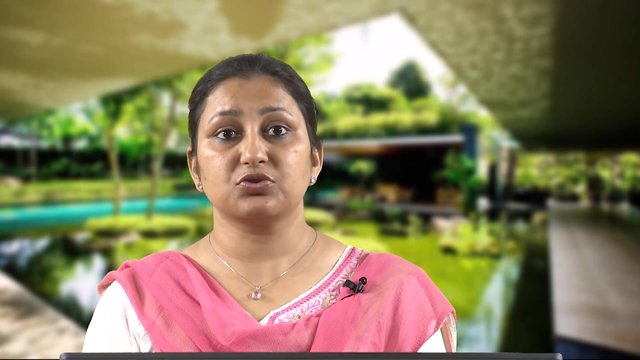 on various parameters. It allows the explanation of the reality, So we have to be able to relate, associate the reality and express it through this model. If it is not doing that, then it is a failed model And it has to represent the systems and is isomorphic to the system. 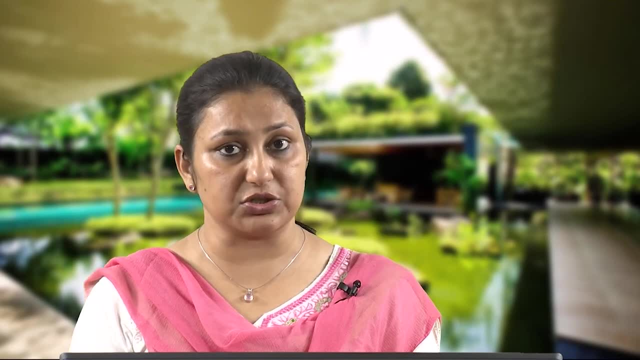 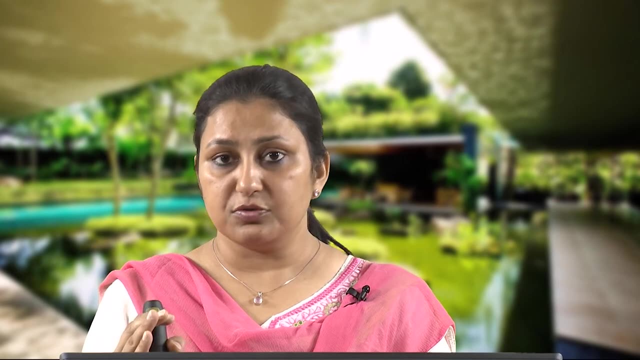 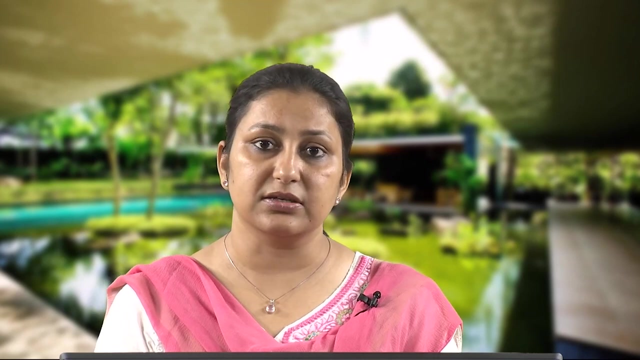 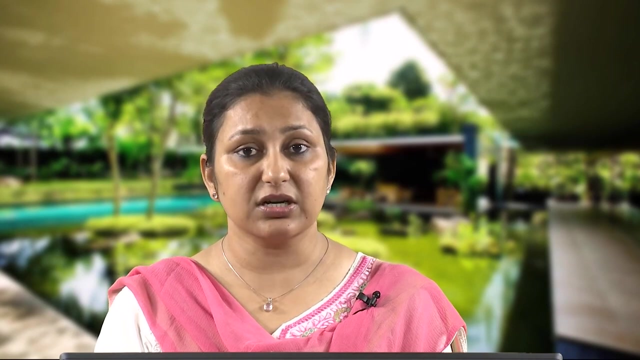 that they represent. So it has to be a direct representation of the reality. Now let us look at some of the models of sustainability. Now, all these different models which are defined to assess, to measure, quantify, define, Understand sustainability can be clubbed under a broad study, which can be, which is termed as: 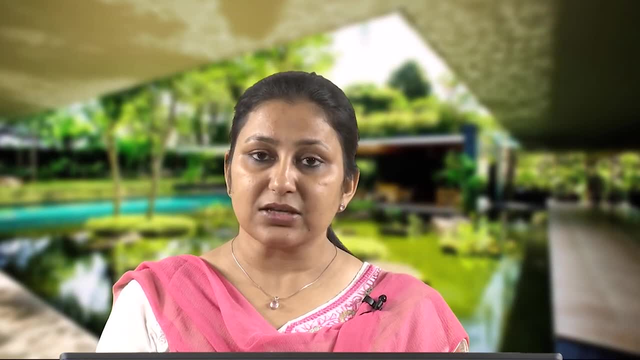 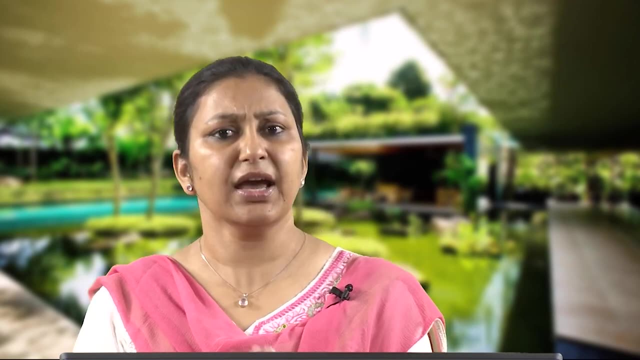 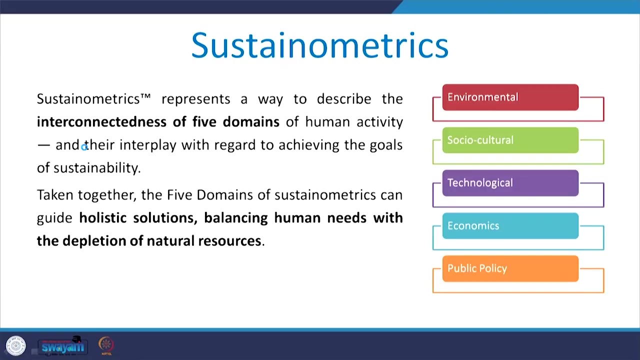 sustainometrics. Now, sustainometrics is actually a way to describe the interconnectedness of 5 domains. So far, we have been talking about 3 domains: environment, society, the social domain and economic. However, if you see, here we are talking about these 5 domains where environmental 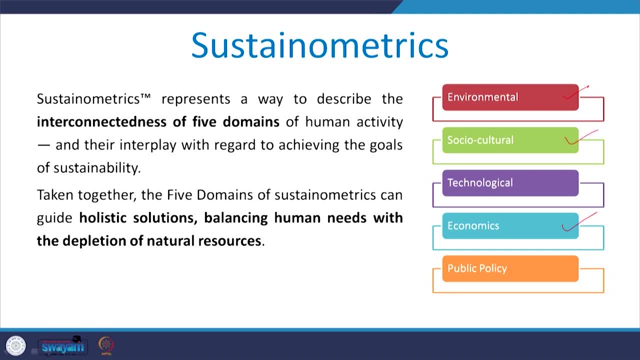 states. socio-cultural dimension is there and economic dimension is there. So the triple bottom line is anyways there. but with given penetration of technology in our life, almost all spheres of life- technology also becomes an added domain and policy, which includes politics as well. So often this public policy and politics 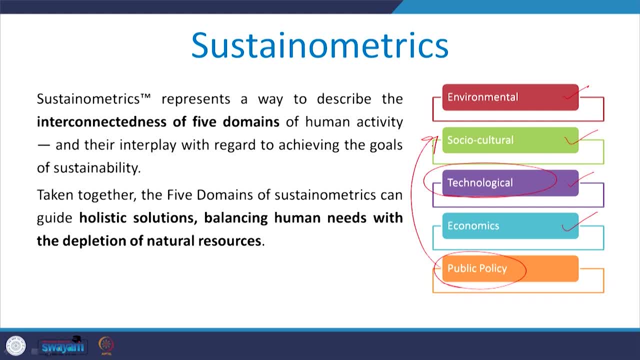 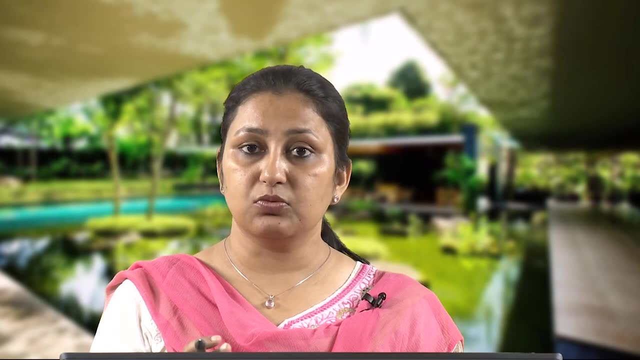 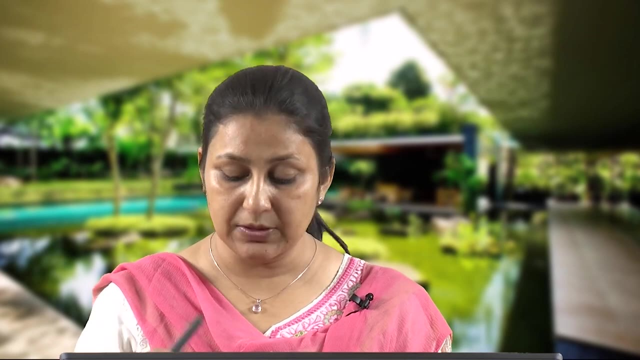 was clubbed within the domain of socio-cultural and gradually it has come out as an independent domain which defines the sustainability, different models of sustainability, Depending upon who is defining sustainability. what is the definition of it? the focus on each of these 5 domains may vary slightly, but they are most likely to be. 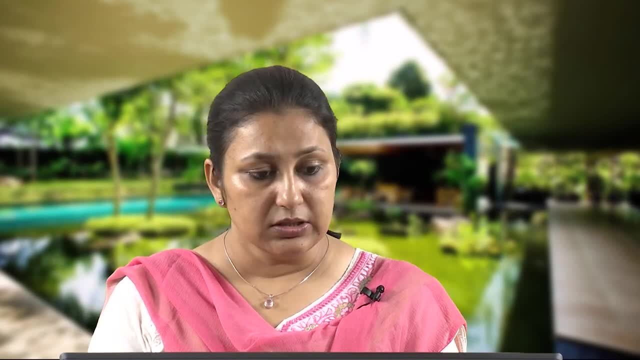 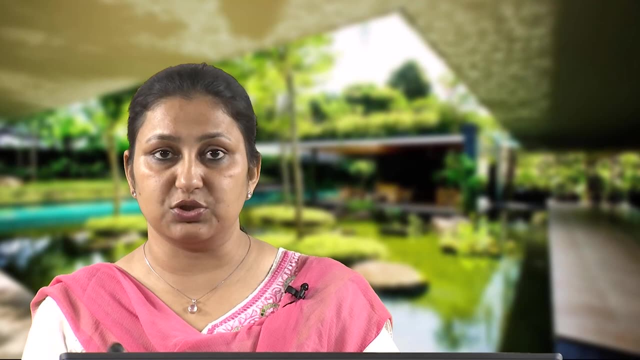 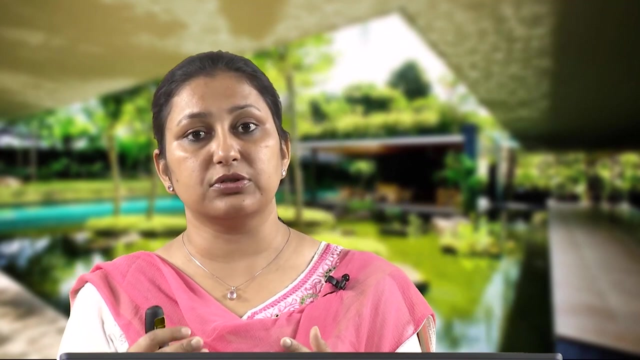 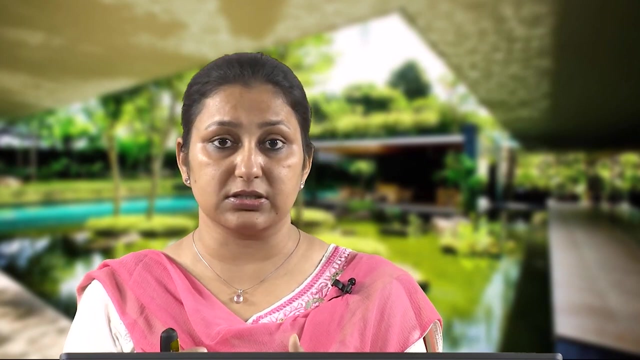 present whenever we are defining sustainability. So what is the criteria for modeling sustainability? Now, sustainability is a very, very vast subject, simply because it encompasses almost everything. We are talking about environment here. we are talking about socio-cultural domain here we are talking about economics. here we are also talking about technology and politics. 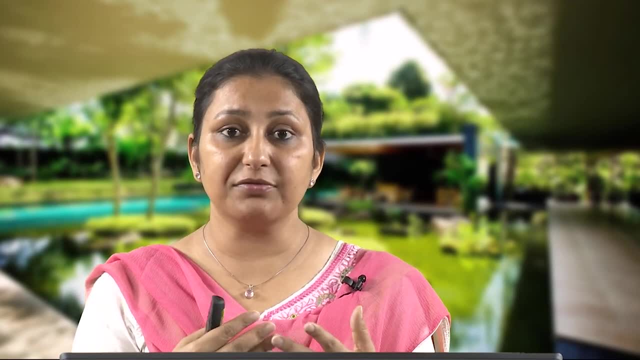 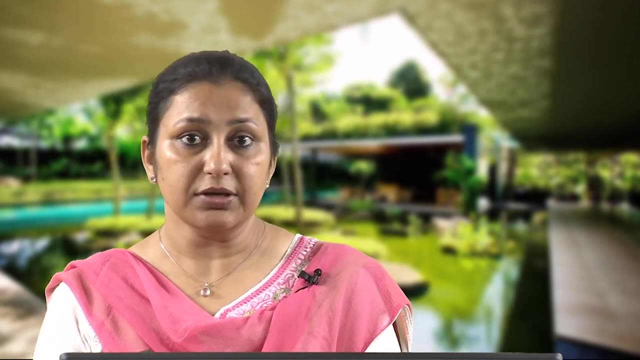 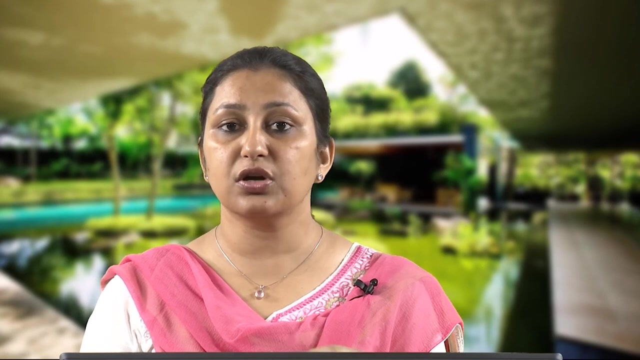 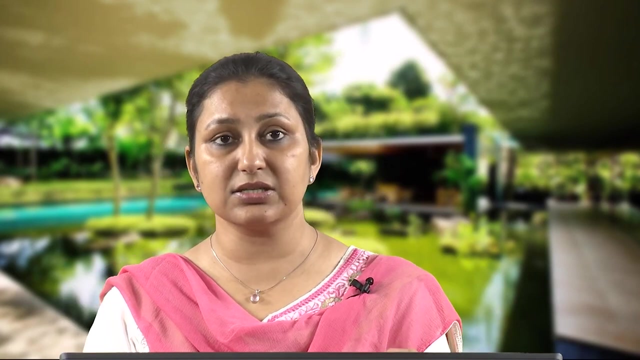 and policies. So it is a very vast domain. it is an interdisciplinary study at any given point of time. So if we are talking about any system from just one perspective, one point of view, it is not understanding sustainability. So the first essential criteria for modeling sustainability is that it has to be interdisciplinary. 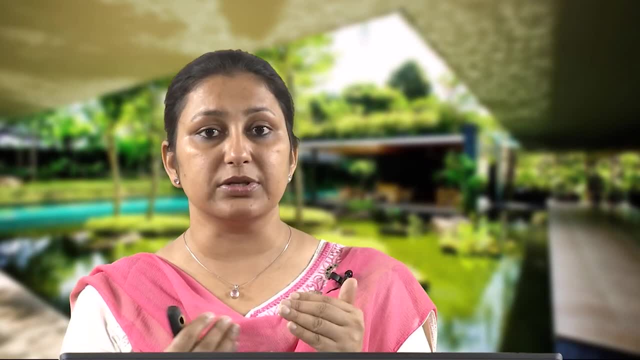 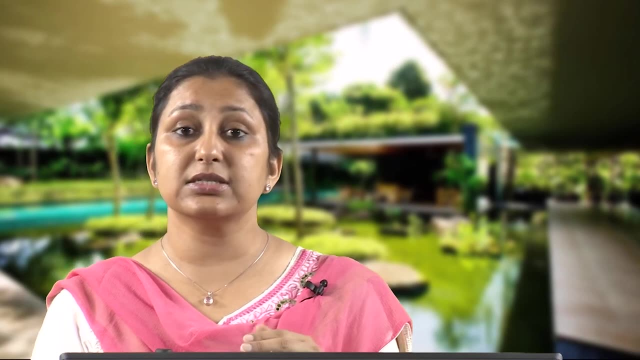 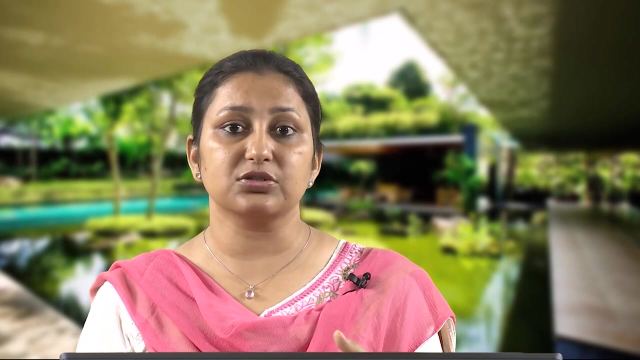 in its approach. It has to talk about all the disciplines, all the domains. Second is it has to manage the uncertainty. Now uncertainty comes in because it is so vast, there are so many domains to be touched upon, discussed about that, there are greater chances of uncertainty creeping in. 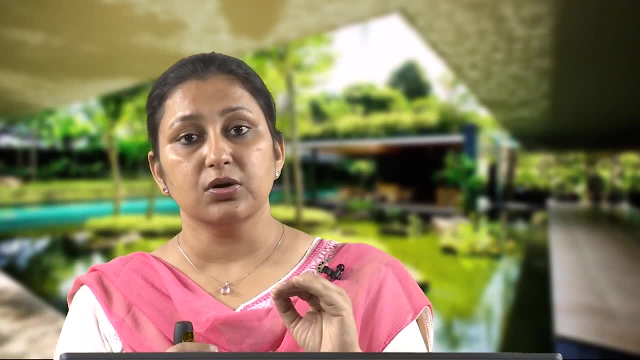 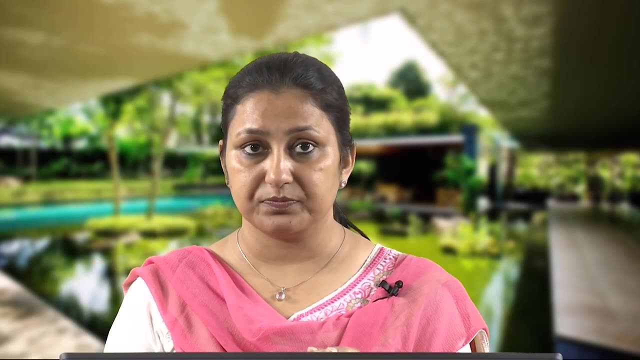 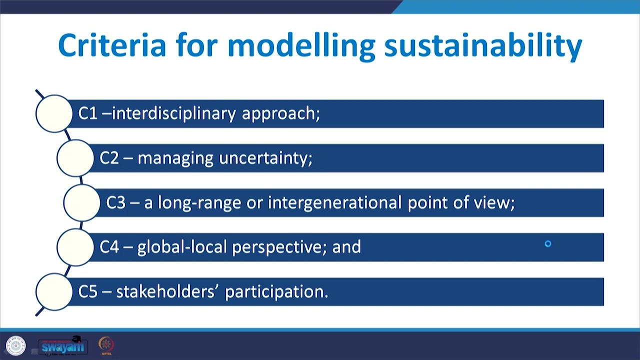 Now, any model of sustainability which we are developing, defining, has to manage that uncertainty in very clear terms. Third, is it has to be a long range or intergenerational, Intergenerational point of view? it has to bring into the picture an intergenerational. 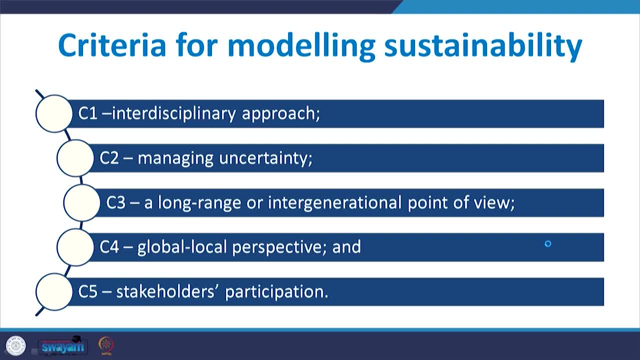 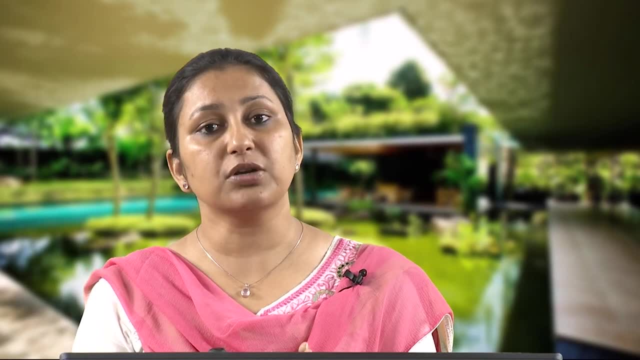 point of view. Now, anything, the moment we talk about sustainability, we are talking about a system to sustain for long, to continue, as we have just seen the definition. So we are not talking in a given point of time, but we are talking about a long duration. 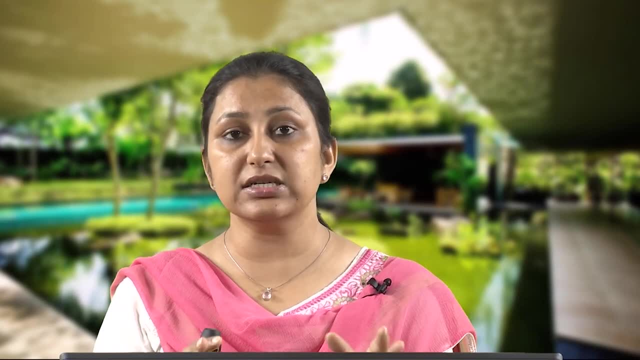 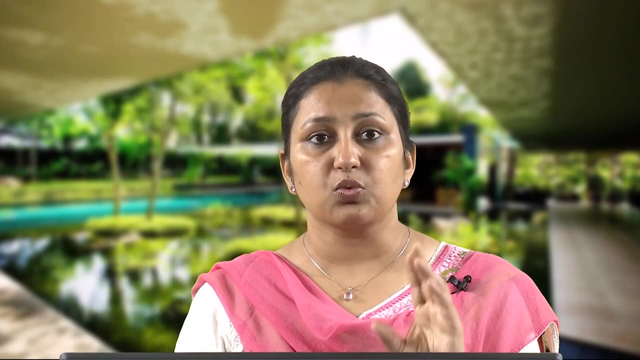 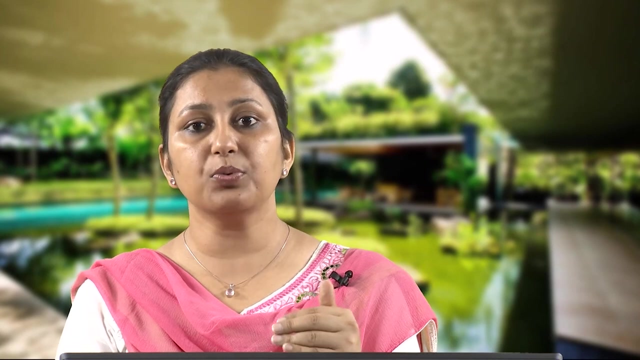 of time And that is why a long range or intergenerational point of view, Intergenerational point of view- is essential to define or model sustainability. Fourth is global local perspective. When we were discussing in lecture 2 that gradually how we are looking at buildings, 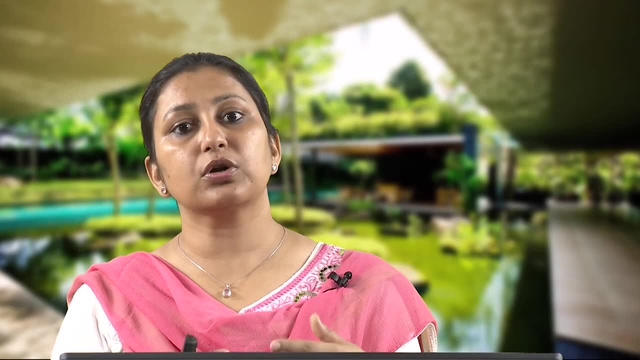 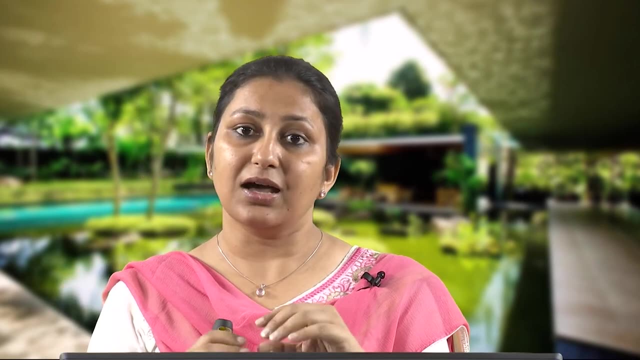 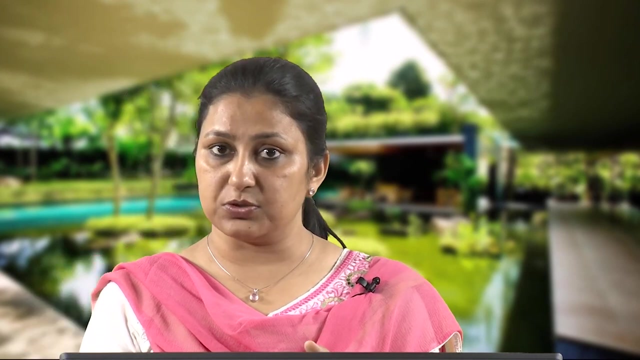 and how we are constructing them is becoming more and more global, while losing the total focus on our local conditions. that is where the unsustainability creeps in, or it becomes the other way around, where we are only focusing about the local perspective. Then also it becomes unsustainable. 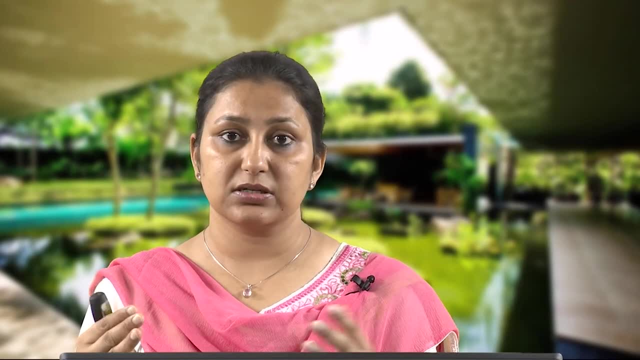 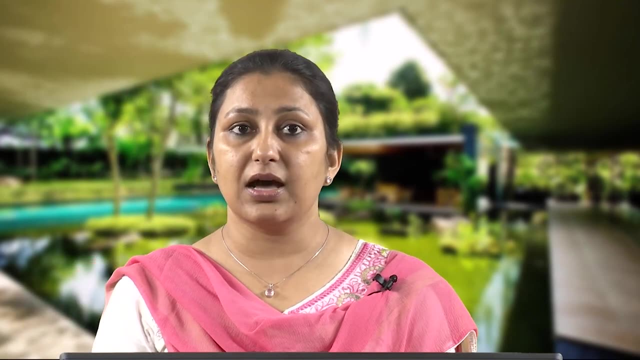 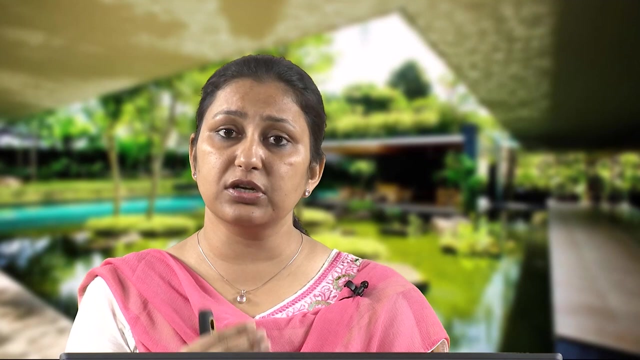 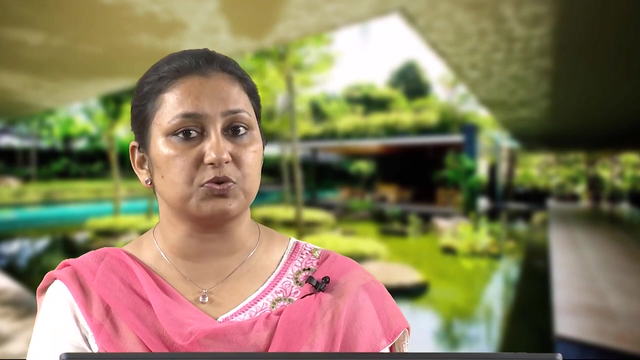 So it has to have a balanced approach where both global and local perspectives are brought together into understanding. And the last is stakeholders participation. We cannot define sustainability or we could not develop a model of sustainability from a third person s perspective. has to incorporate the perspective and participation of the stakeholders. 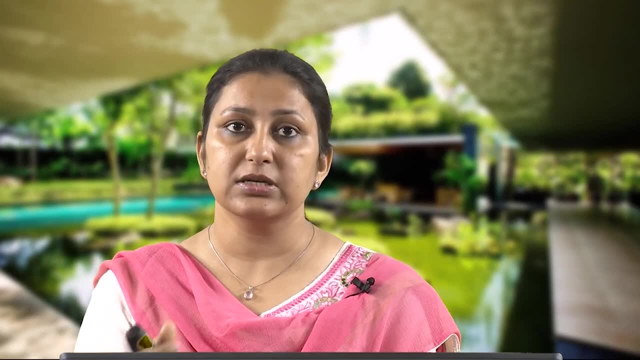 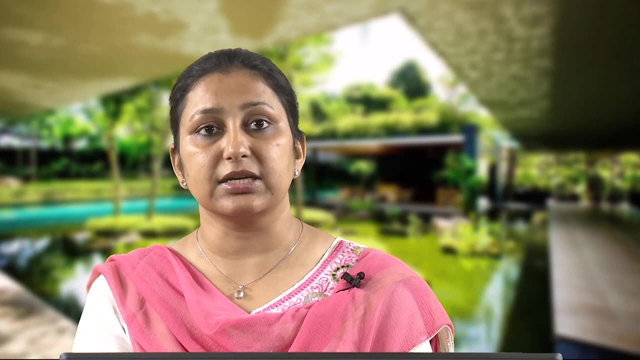 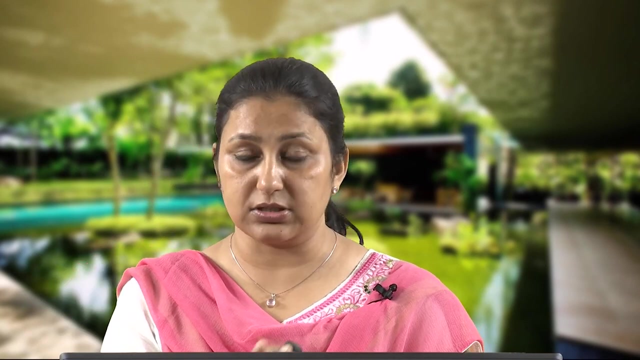 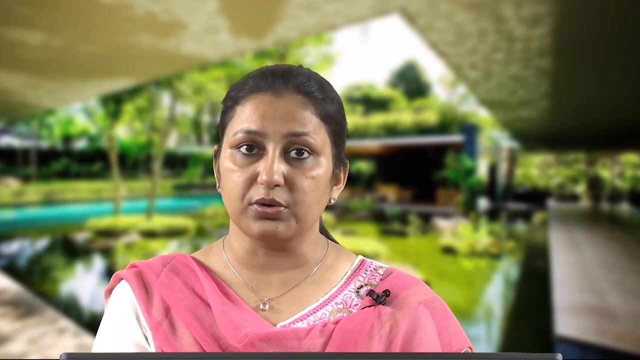 who own that system which is being tested for its sustainability. So, with these defining of criteria for modeling sustainability, let us look at the different types of models of sustainability which are available as on date. So people have tried to define sustainability through different types of models. One is pictorial visualization model. 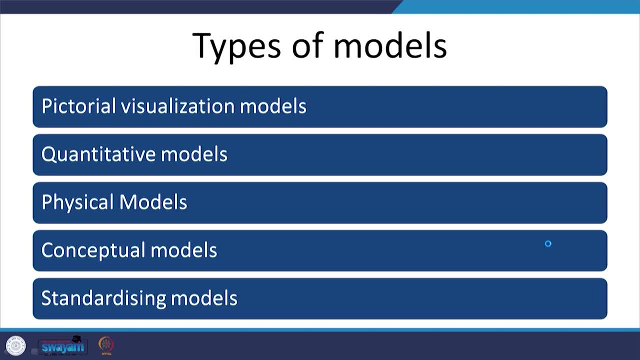 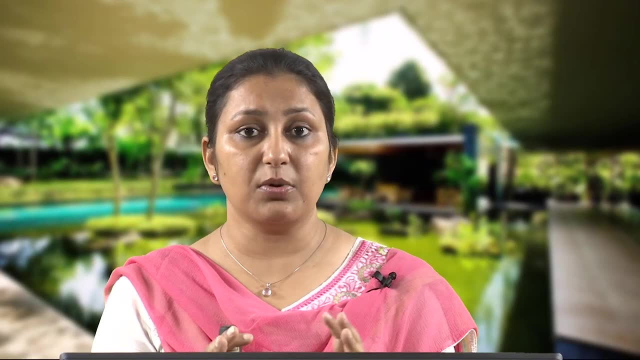 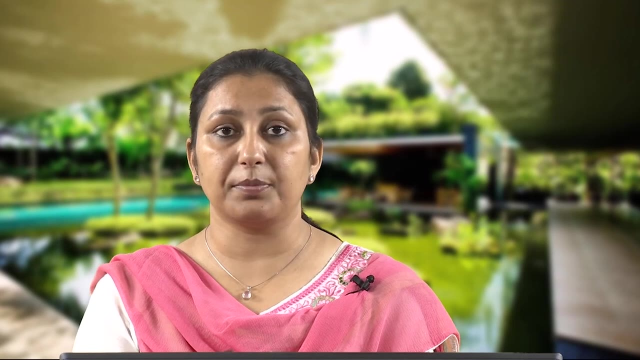 Next is quantitative model, which talks about numbers and quantifying, measuring the different parameters. Physical models which are physically available, which are tangible, which can be seen constructed. Conceptual models which are available only as a concept, and standardizing model, where we develop standards And talk about sustainability. Let us look at each of this model and briefly discuss about. 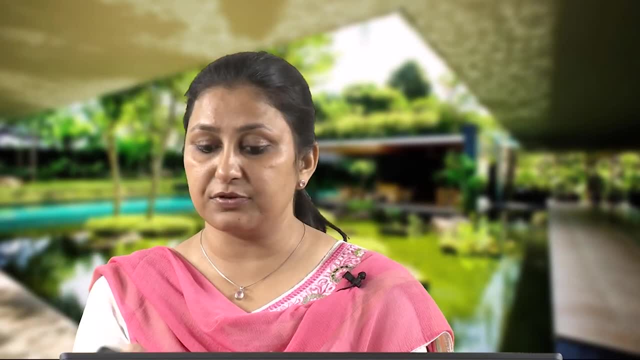 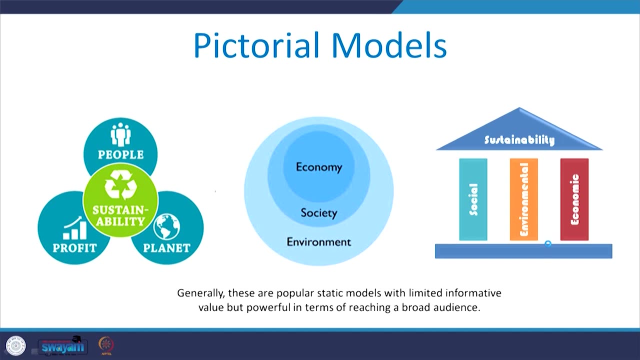 what we understand by sustainability through these different types of models. Now, these models, this pictorial model- here This we have seen, which was the first representation of sustainability through the Venn diagram. Now, gradually, people started arguing that what is the use of? 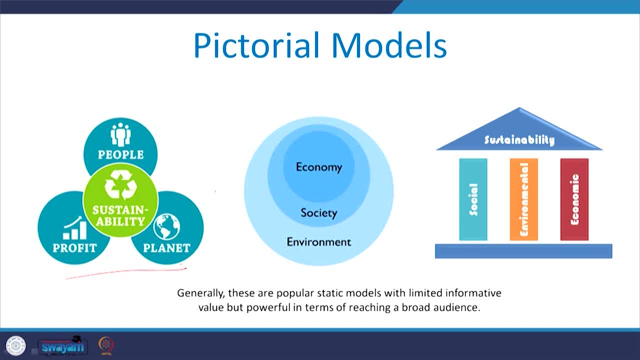 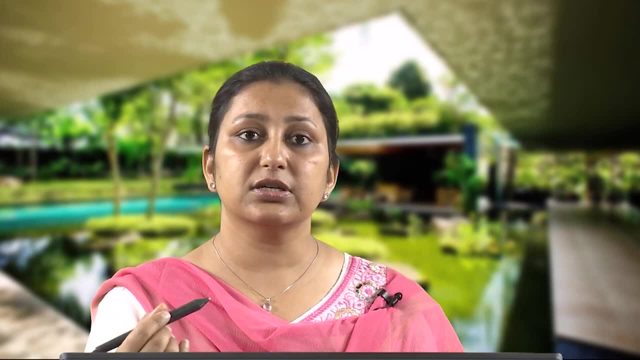 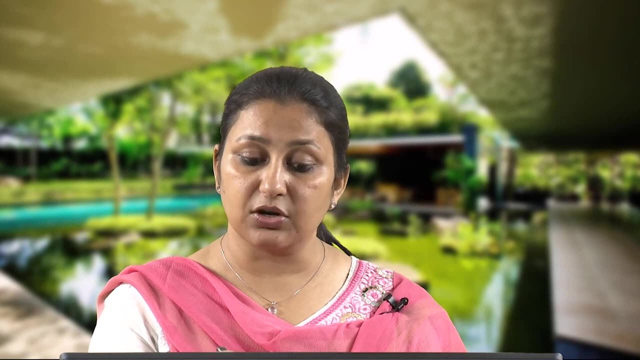 economy if the environment is not there. So there was one very noted ecologist, environmentalist, Herman Daly, and he discussed what is the use of a sawmill if the forest is gone? So what is the use of a sawmill, which is used for generating economy, if the 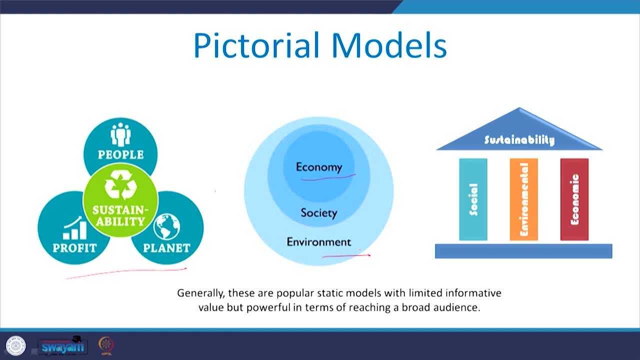 environment is not there if the forest is not there, and that is true for all the cases. So the definition of sustainability through the pictorial means was redefined, where environment Environment would become the main focus and the larger point of discussion, while society and economy are within the environmental 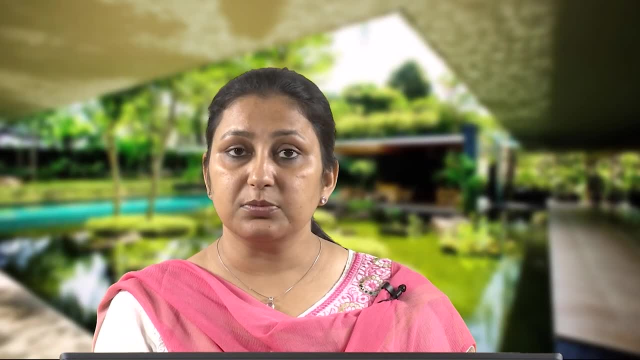 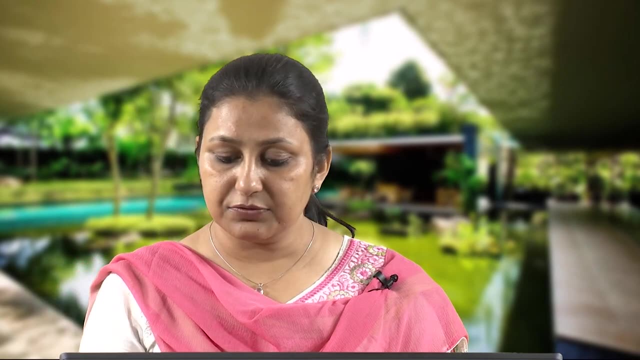 domain. So the definition of sustainability itself changed, evolved, where a larger emphasis was to be placed on environment, Another definition where sustainability was supported by these 3 pillars which we have seen so far. All these 3 pillars were just three pillars. They are place atmospheric. 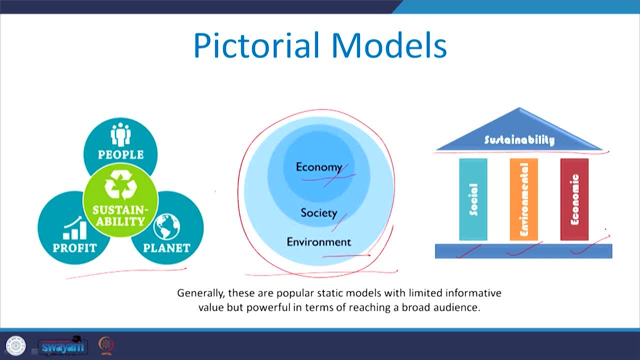 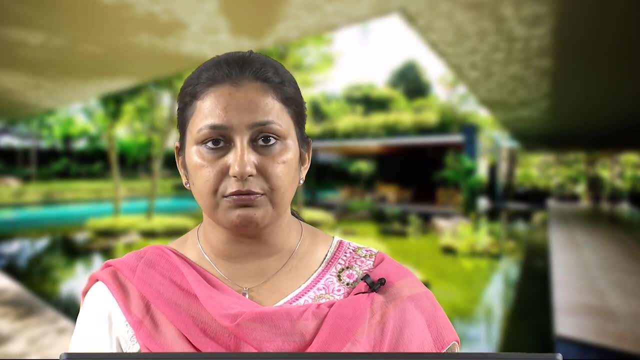 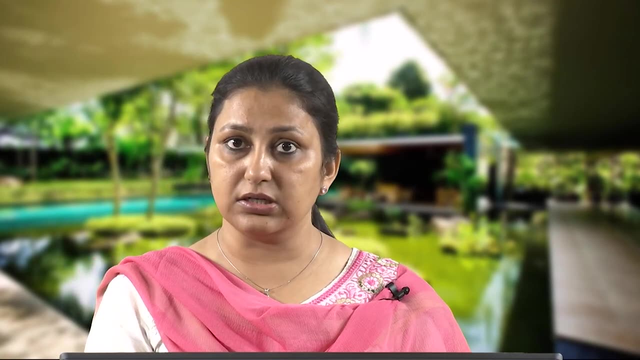 環: agricultural and climate versus industrial sustainability. These were 3 hear's purposeful studies. three domains was also developed. Now all these pictorial models essentially discuss about a very broad understanding of sustainability. Now, from these models we cannot really quantify or understand a given context very clearly. 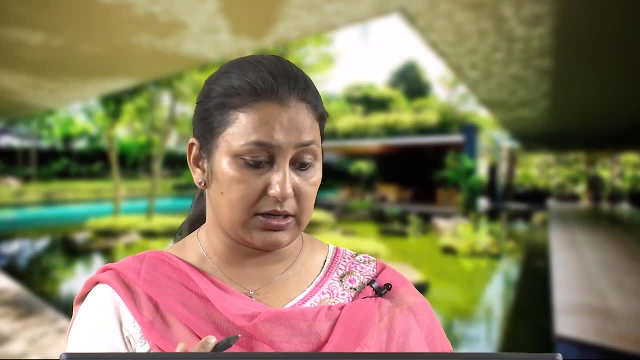 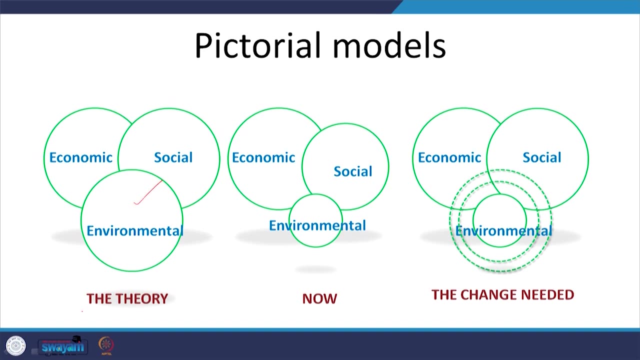 but we can make a form, a general understanding. Now these models have also been changing. for example, initially we were talking about this theoretical model where we considered all these three spheres to be equal in size. Currently there is a larger focus on economy, so the environmental, the focus on environment. 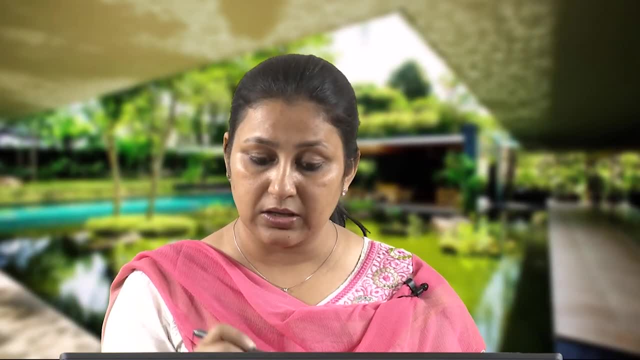 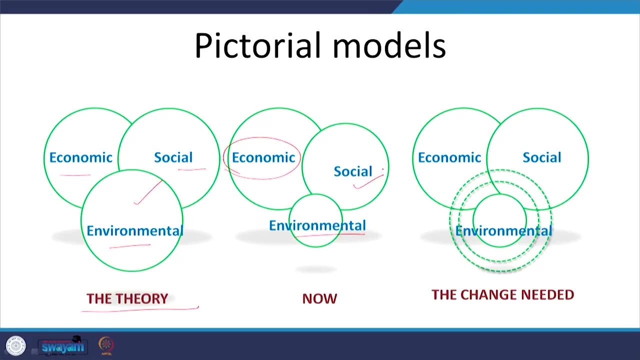 has been decreasing. it has been greatly reduced and the social sphere is where it was. However, the kind of change that is required to sustain the world at large is that the environmental sphere grows bigger And the other two spheres, if not diminish, they remain the same focus. 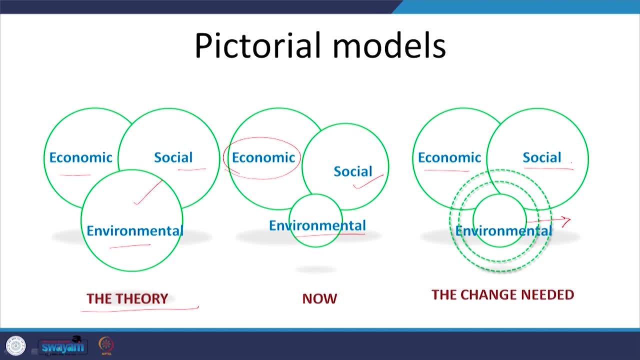 So this is the kind of understanding we get through pictorial models. Now, how will this be done? How will the environmental sphere be enlarged? What do we mean by enlarging the environmental sphere? All those things may not be understood through a pictorial model. 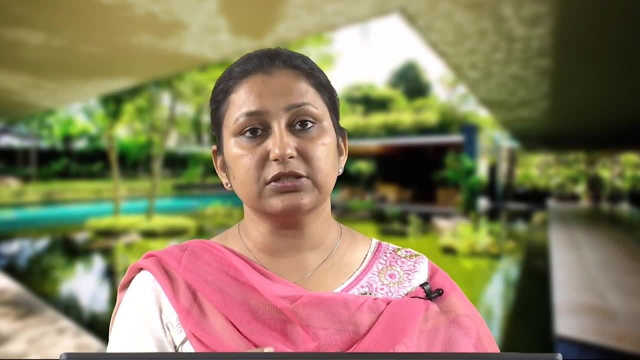 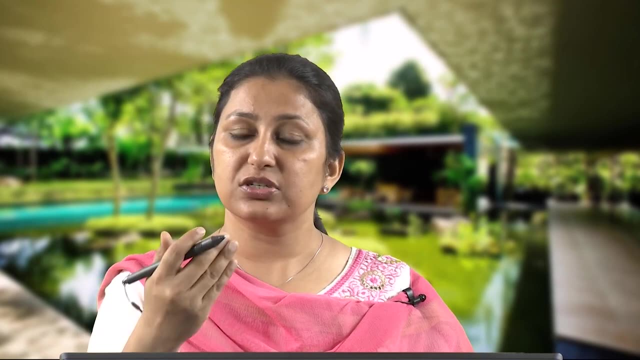 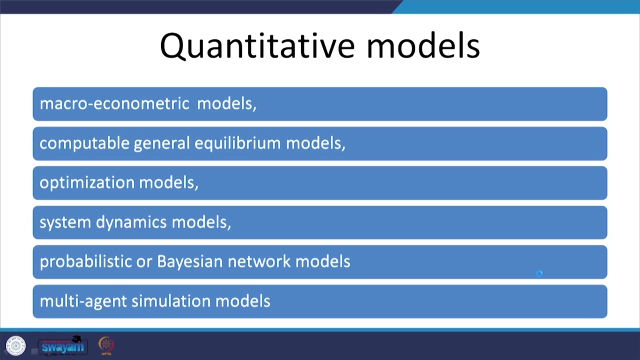 Next we can come to quantitative model. now quantitative model is a type of model which quantifies the different parameters which lead or which impact sustainability. There are different types of models within quantitative macroeconomic model: computable general equilibrium model, optimization model, system dynamics model, probabilistic models. 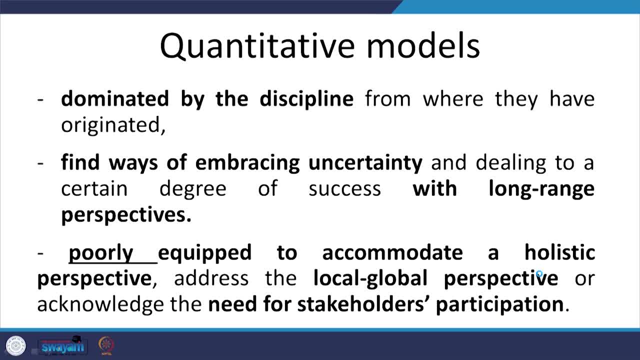 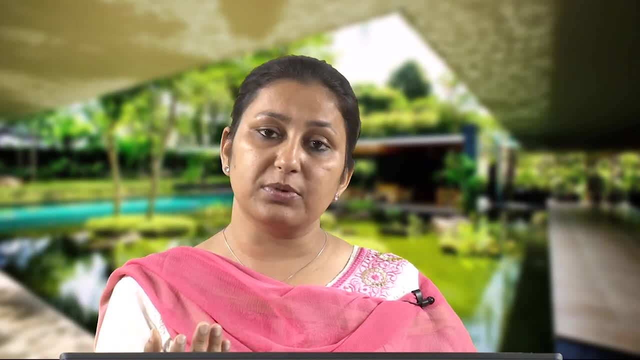 and multi-agent simulation models. We can quickly look at these, but the basic quantities of quantitative models remain the same. 1. They are often dominated by the discipline from where they have originated. So if they have originated from the economic discipline, we would always find larger focus. 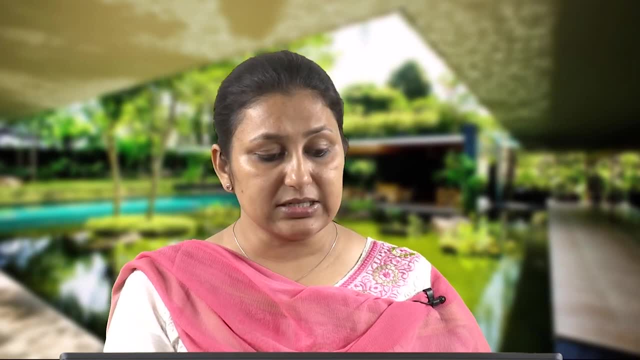 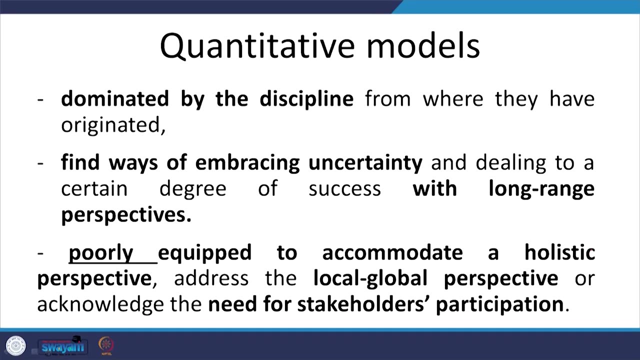 of the economic discipline and like that. 2. Second is, they find ways of embracing uncertainty quite well, and to a certain degree they also deal with the long range perspective, because they put the numbers into it with the help of these different parameters. 3. 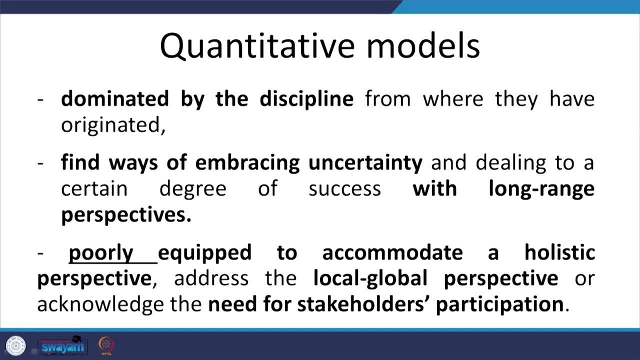 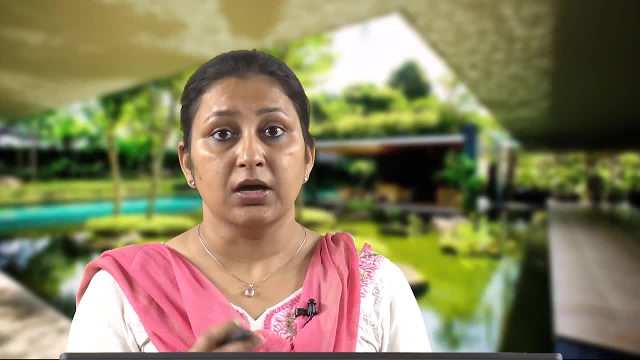 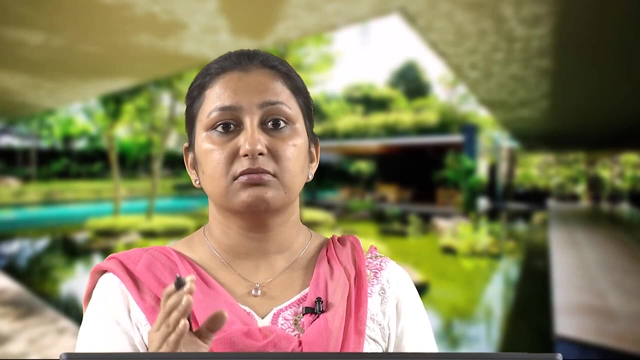 However, the drawback is that they are poorly equipped to accommodate a holistic perspective, because it is not possible to take into account all the parameters which affect sustainability of a system, of a model, and they are poorly equipped to address the local global perspective often, and they do not often acknowledge the need for stakeholders participation because 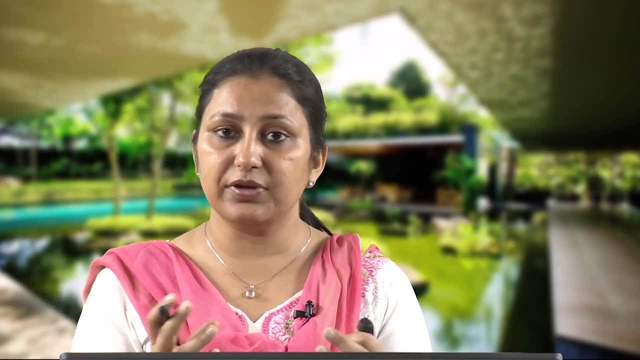 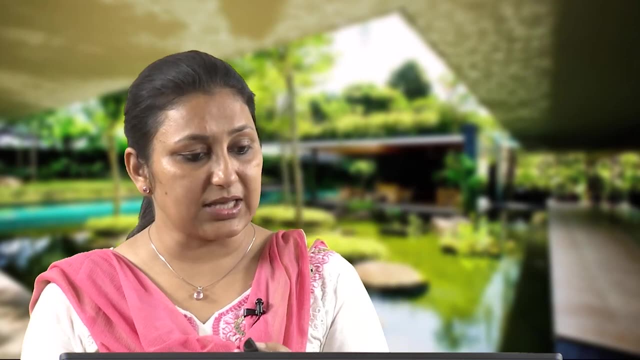 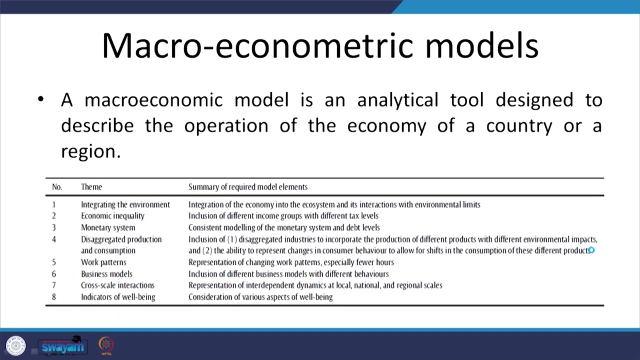 these parameters are so quantitatively dealt that we are only looking at the numbers, but we are not looking at how stakeholders are responding to it. Some of the examples are, say, one of the macroeconomy trick model actually talks about the operation of the economy of a country or a region by taking into account these different parameters. 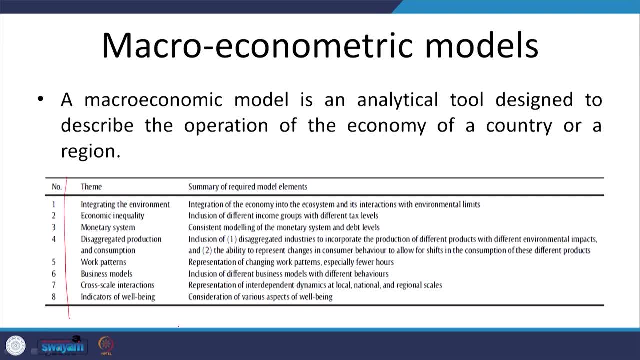 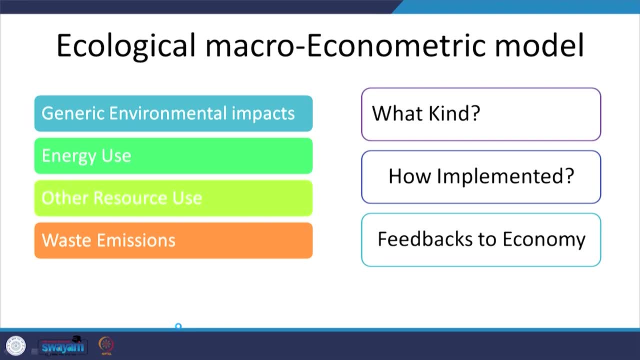 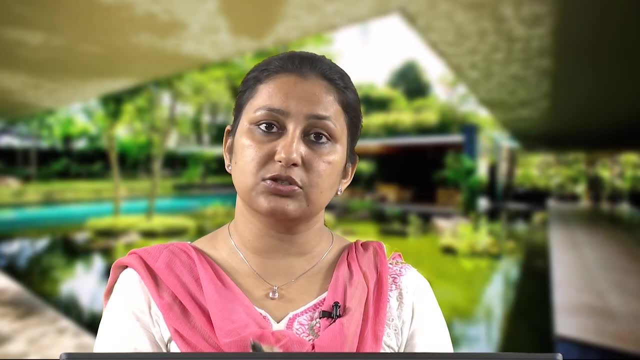 these different themes, incorporating them 4.. However, the focus on these themes may vary little bit. The next is ecological macroeconomy trick model. It is the subset of macroeconomy trick model where a larger focus is on economy of a country. 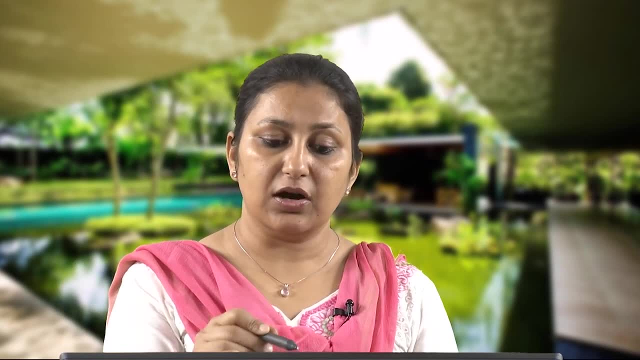 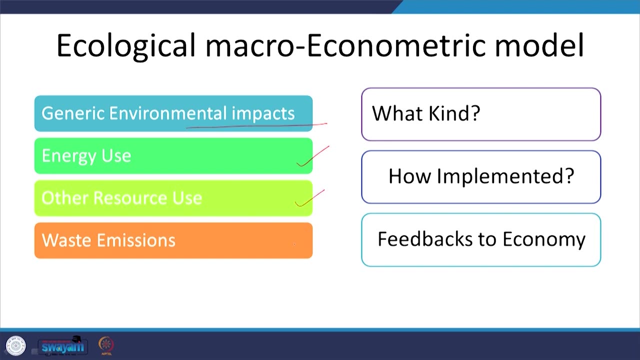 or a region or a place, but we are talking about the generic environmental impacts. We are talking about, say, energy use, resource use, water emissions, and all of these in terms of economy. So we are talking about their impacts through a feedback on economy. 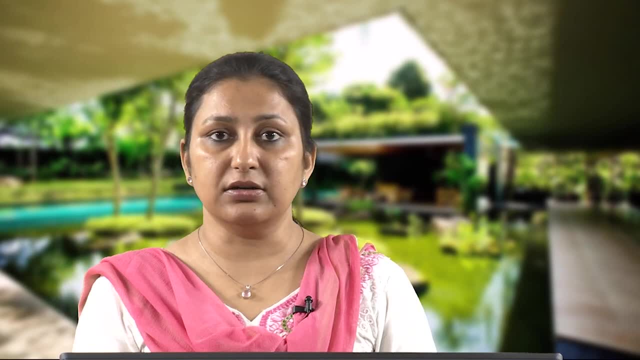 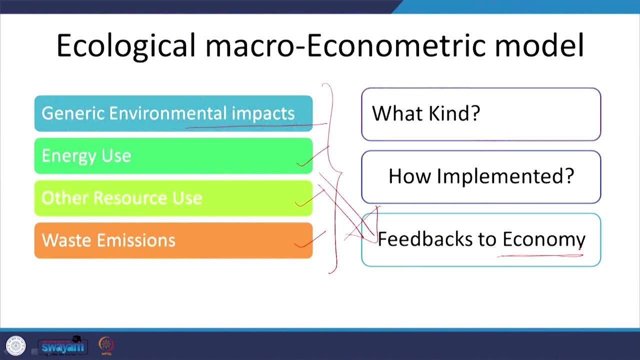 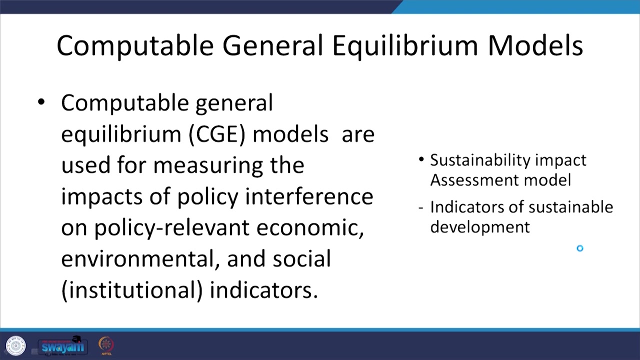 So if a place, if a country implements, say, a particular policy or a particular program or system is being run, how is it affecting the economy will be tested, and that is what this ecological macroeconomy trick model does. 5. It uses computable general equilibrium model which are used to assess the impact of policy. 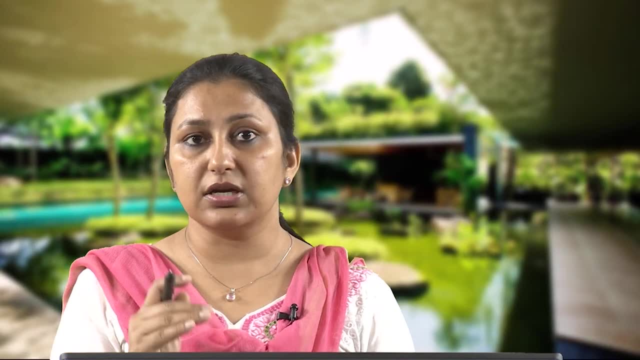 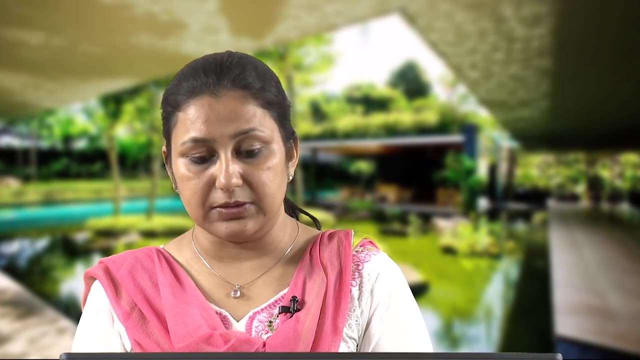 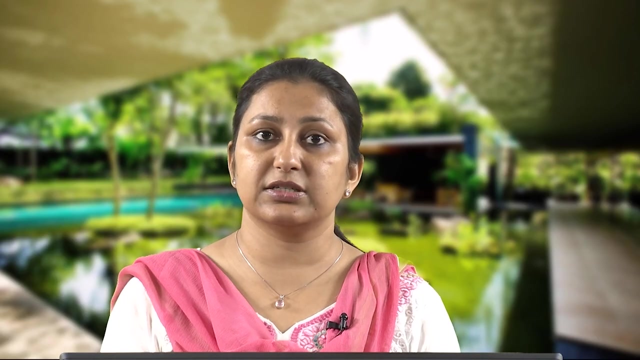 interference of policy relevant economic, environmental and social indicators into one model. For example, we have a policy, say government of India comes up with a policy that every village gets connectivity of pucca roads, permanent roads 6. So we have a policy, say government of India comes up with a policy that every village 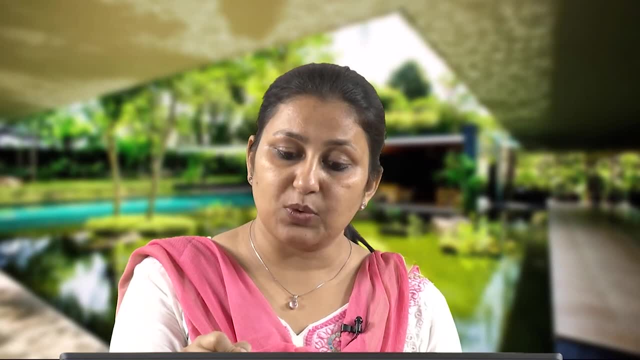 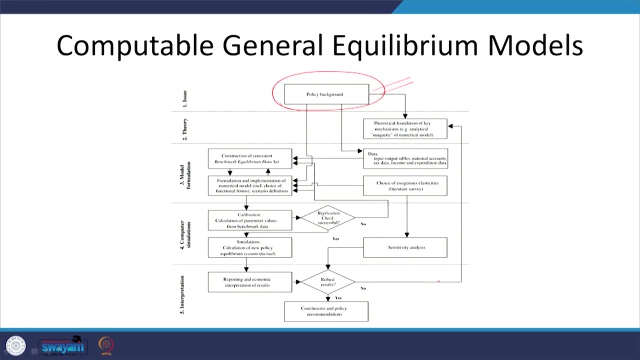 gets connectivity of pucca roads, permanent roads. Now, this is one policy. now, what is going to be the impact of that policy will be understood through this computable general equilibrium model. Now, here we will be talking about the environmental impact of it. how much material will be required? 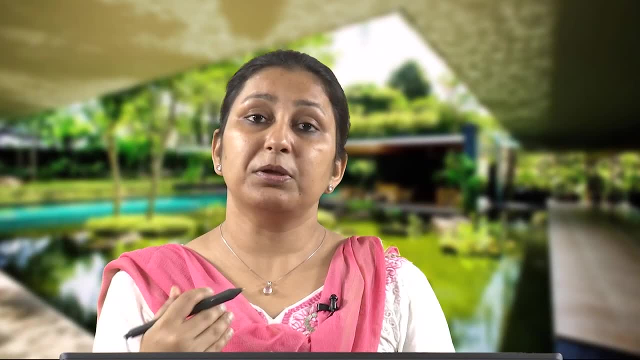 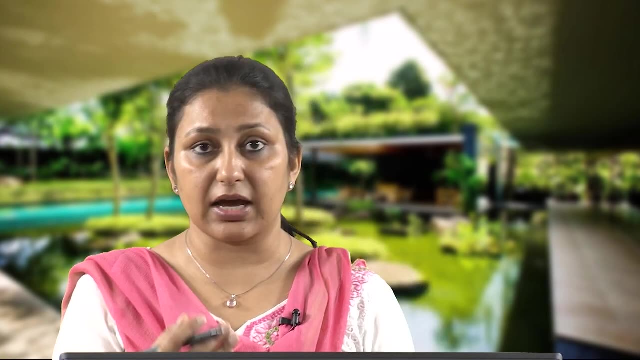 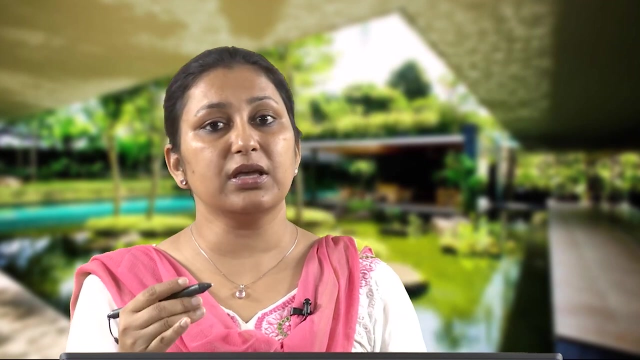 there will be a social impact of it. that. how, when people are connected through roads, how will they be benefited? they will have better access to medical facilities, they will have better access to education. So that is a social impact of the same policy and there will also be an economic impact. 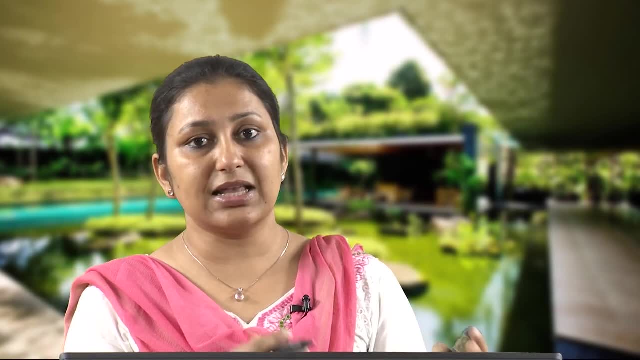 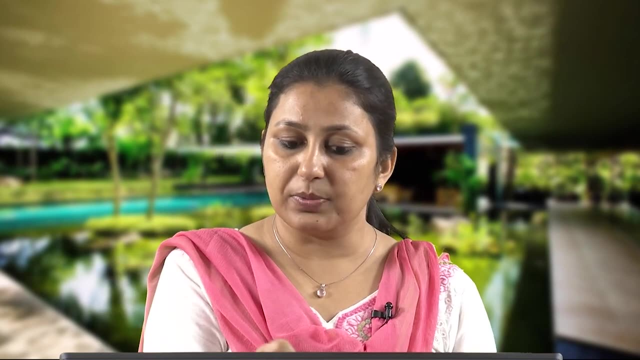 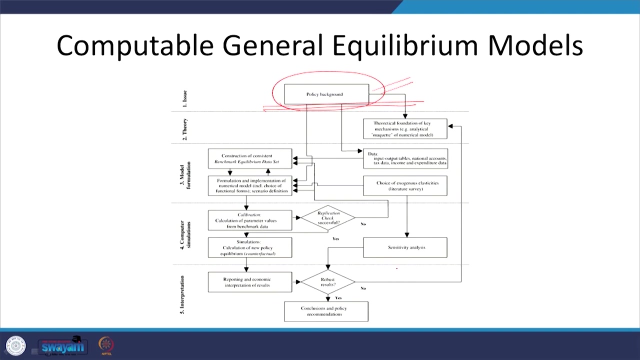 So the farmers in the villages will be able to sell their produce for a better price when they go take their produce to the cities. So a policy will be taken up and its impacts will be calculated through these different parameters. and finally, the conclusions of. 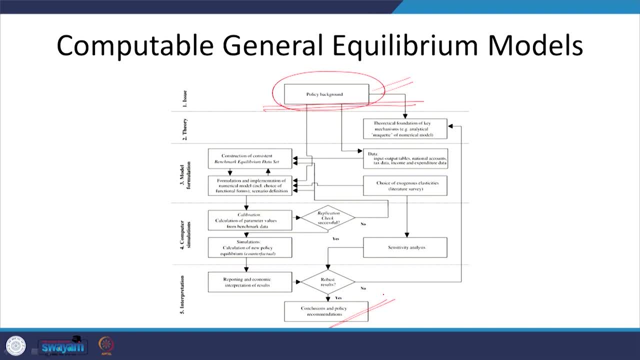 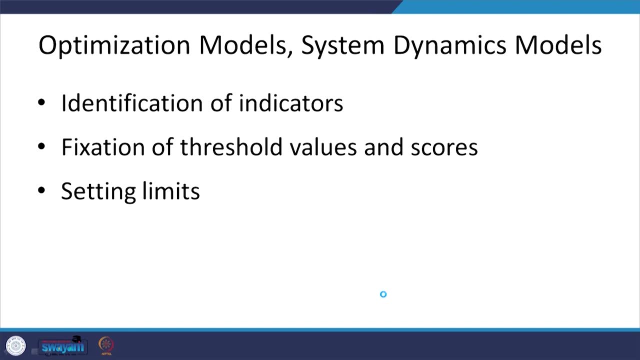 7. And recommendations for the policy will be made. The next is optimization model, or system dynamics model. now here it largely relies on identification of indicators. Now suppose if the indicators have not been properly identified, the system dynamics model may fail because it is not even considering a particular indicator. 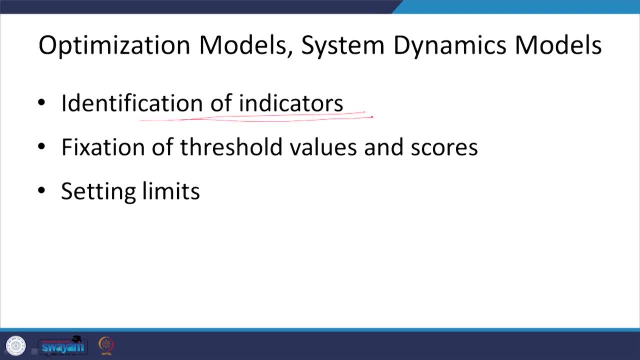 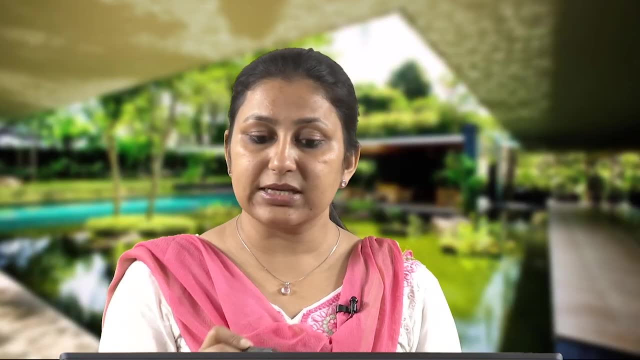 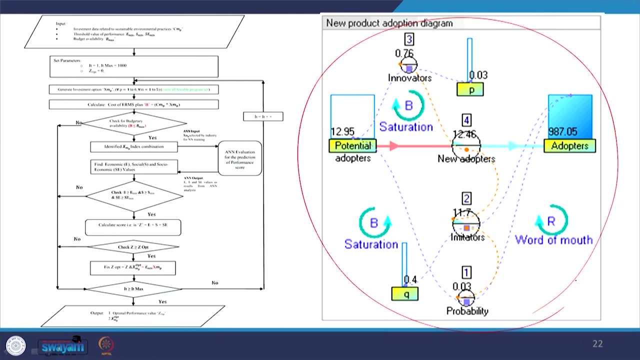 However, if the indicator has been aptly identified, clearly identified, Then, based upon the data analysis, data acquisition and data analysis, a robust model can be developed which will explain the interdependencies of a lot of different parameters and it will explain- it can explain- sustainability to a large extent. 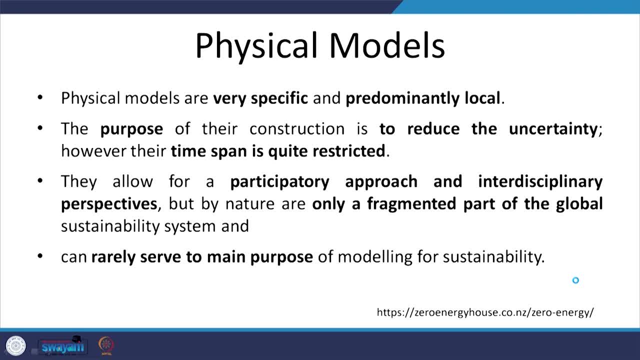 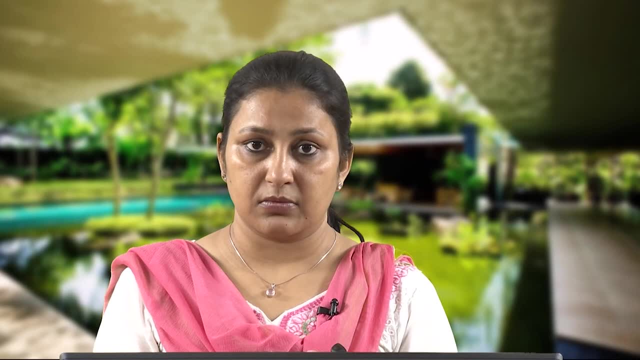 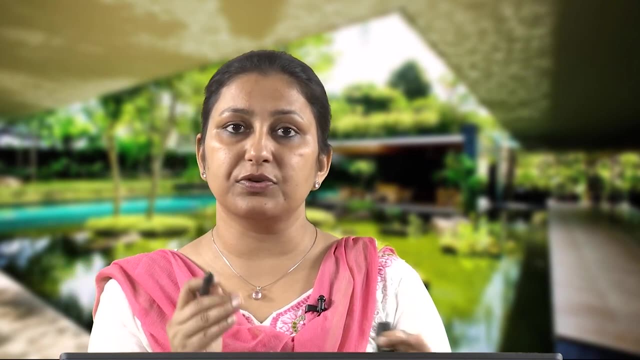 These were all different types of quantitative models. The next type of model is a physical model. Now, physical model, as I said, is a tangible model, a real model which we can see, For example, model of a net zero building. Now, there we will be constructing a net zero building, a model of it, a physical model of. 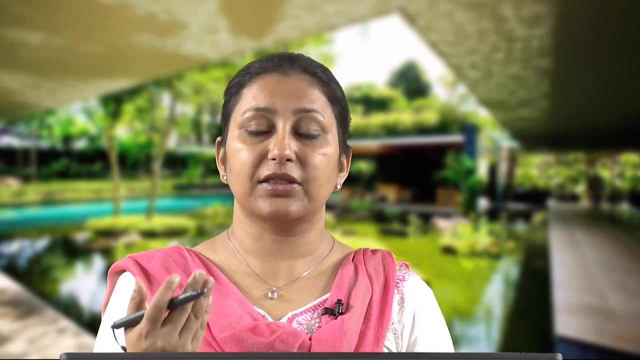 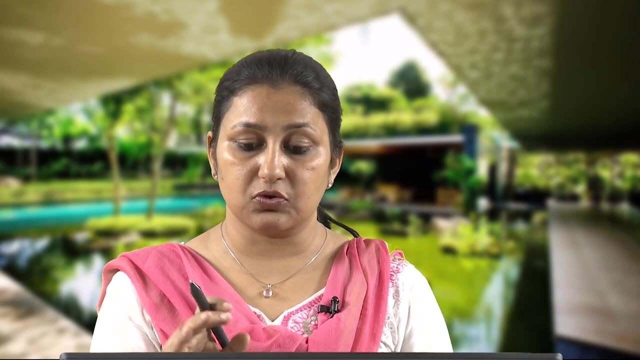 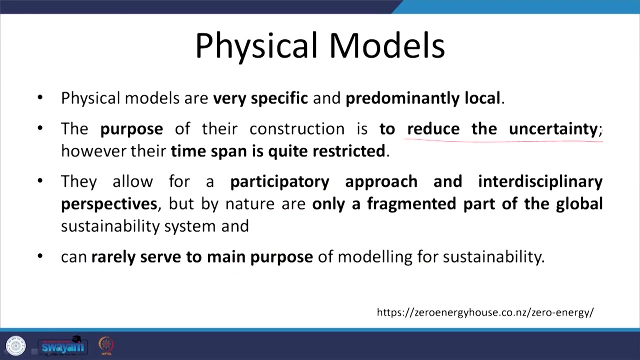 it and then carrying out tests, gathering data based upon that physical model. It is very specific and it is largely local. So there are certain drawbacks, because it, yes, reduces the uncertainty to a large extent. However, the time span is quite restricted because we are talking in a 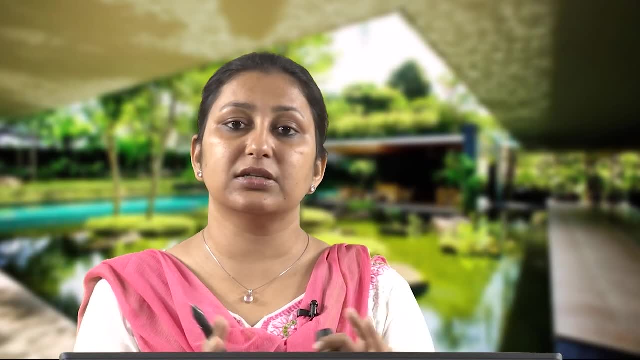 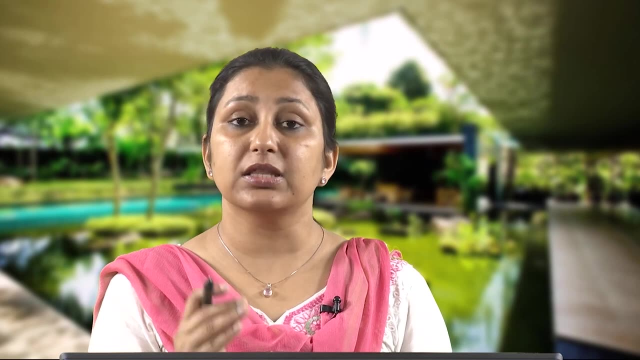 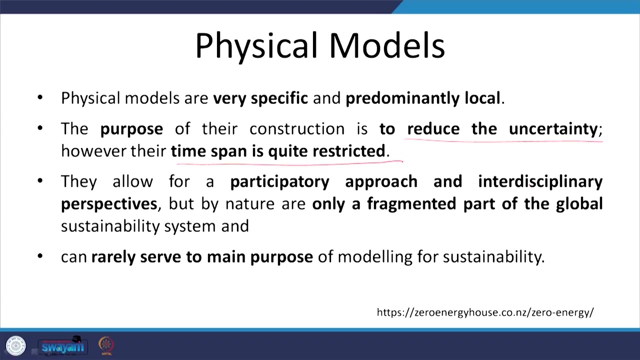 moment of time. The model was constructed today and the tests were carried out today, So the results are also valid for this given span of time. They may not be long ranging. Another: they, yes, allow for participatory approach and interdisciplinary perspectives. 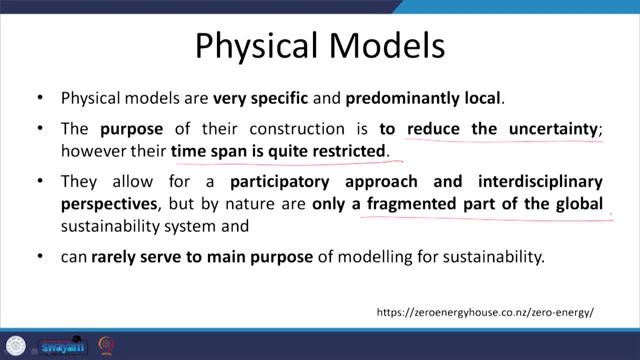 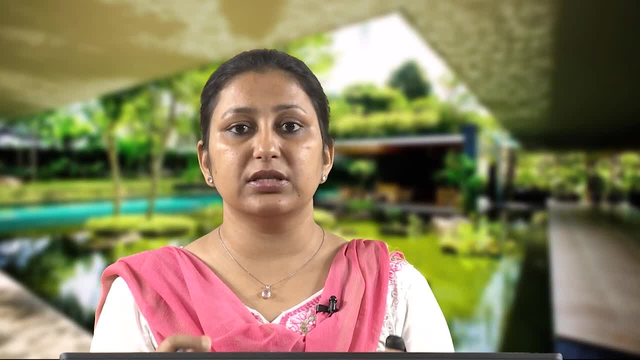 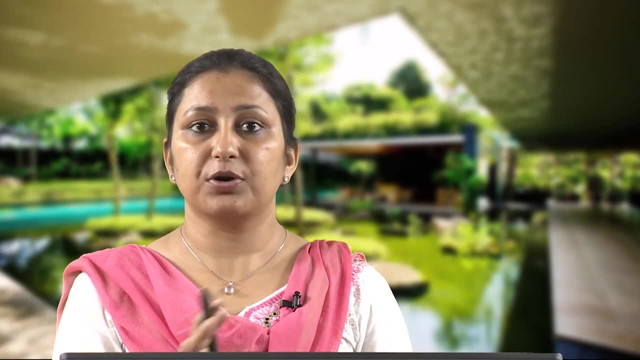 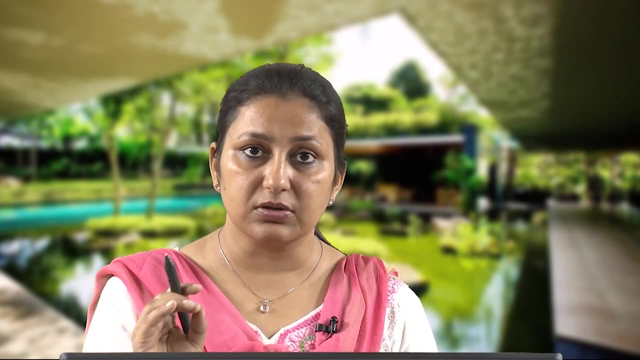 but they are only a fragmented part of the global sustainability system. simply because they are so predominantly local and confined within the time and space, They are very rarely used to serve the main purpose of modeling for sustainability. They largely cater to the requirement of ruling out the uncertainties for a very specific issue. specific problem: 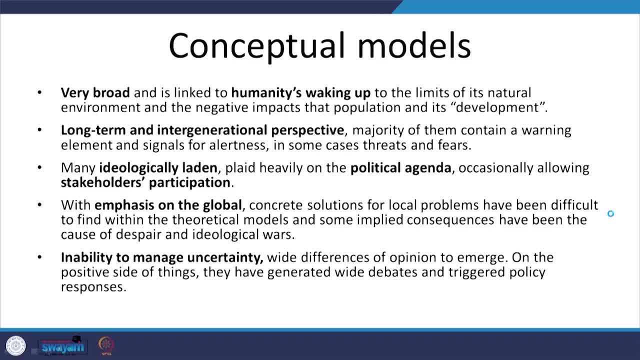 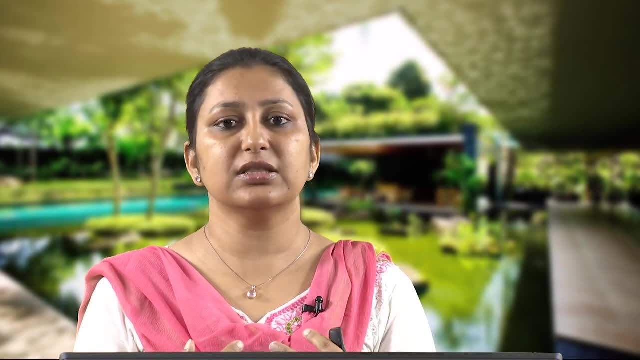 Say, for example, I said net zero buildings. The next type of model is a conceptual model. Now, conceptual model is a very broad model and it is largely linked to very grave, serious issues which concern the entire world globe, humanity at large. 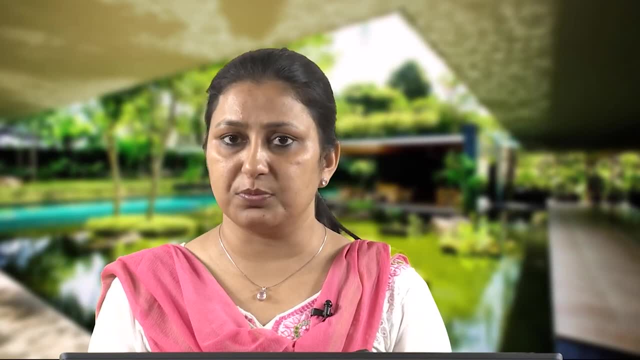 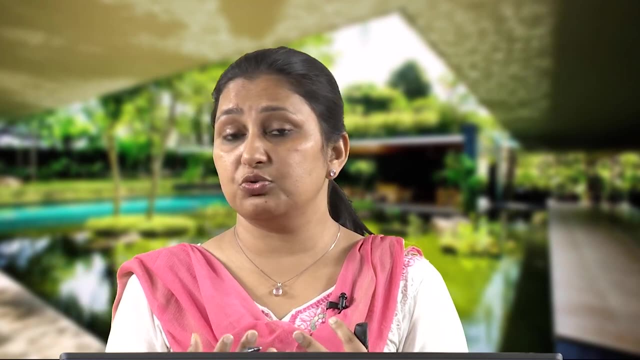 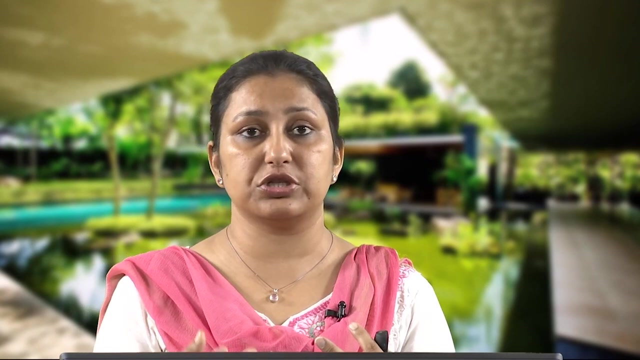 And they talk about the long, long term and intergenerational perspective. They are not locally focused. We are talking about global issues, global perspectives. They are usually ideologically laden. They are heavy on ideology. People talk about ideologies through these conceptual models and it largely is driven. 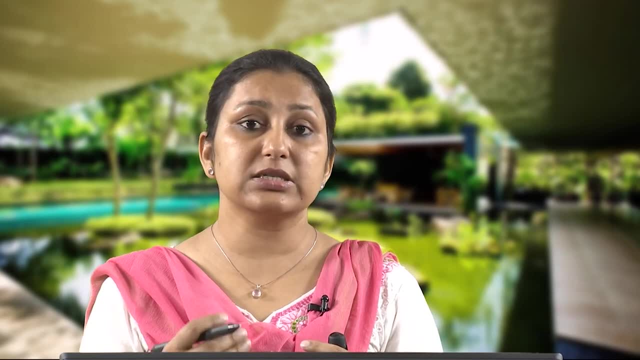 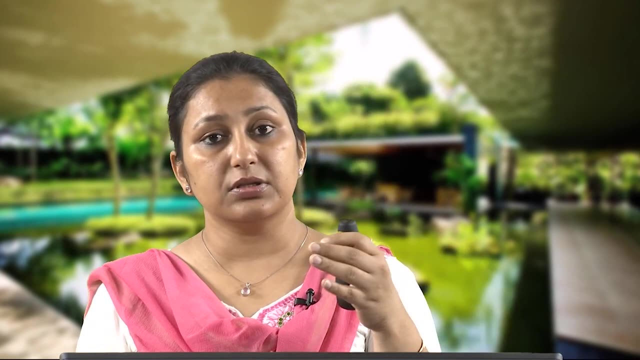 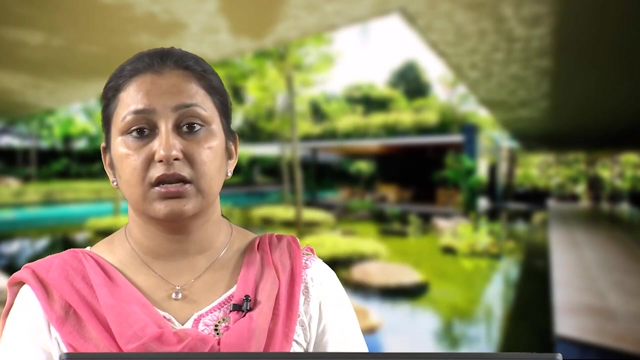 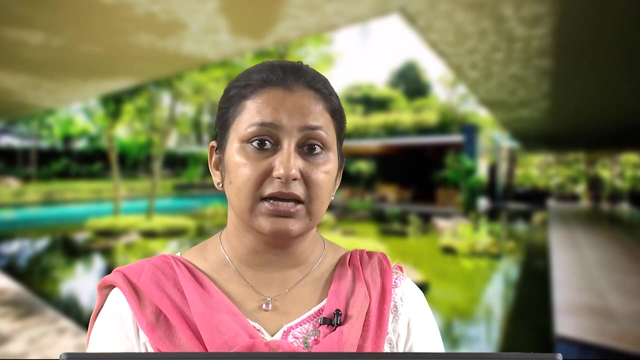 by heavy political agenda. So politics is driven through these conceptual models. Let us look at one of the examples. For example, the entire conceptual model of ozone depletion. so at that point of time when the depletion of ozone was brought to the forefront by scientists, at that time enough scientific 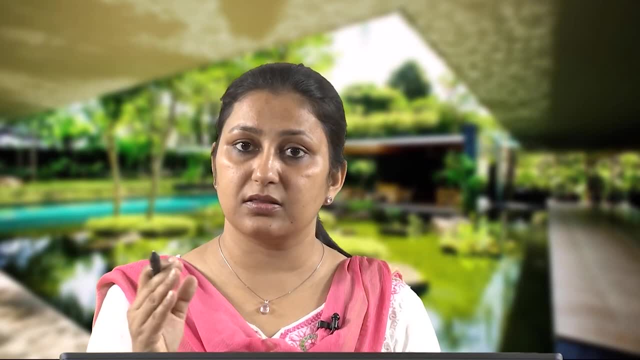 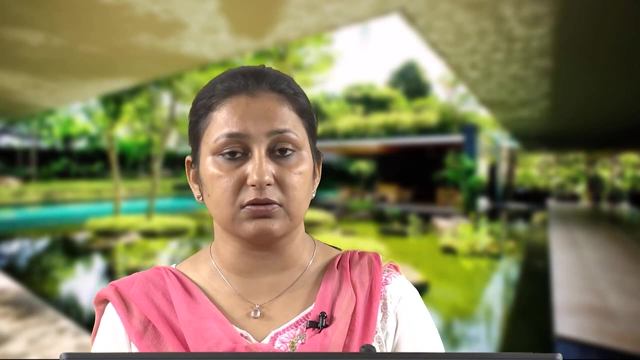 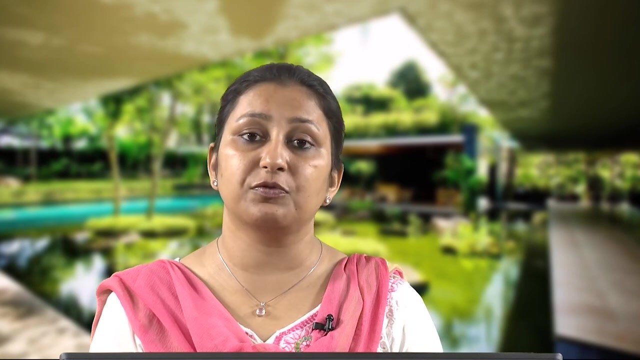 evidence was not available to back the fact or to back the point of discussion whith towards that ozone depletion is happening at a very fast pace, Scientists said. when ozone debt is brought to the forefront by scientists, Scientists did not even know for sure with conformity that what is causing the ozone. 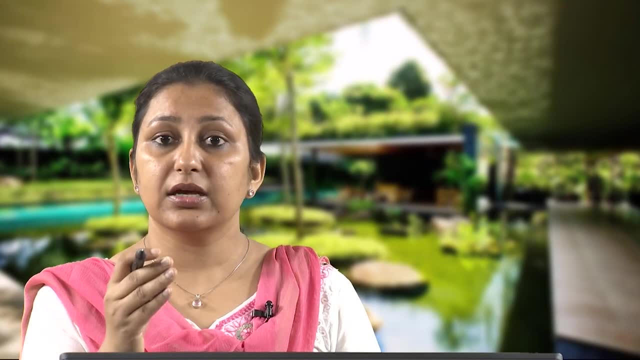 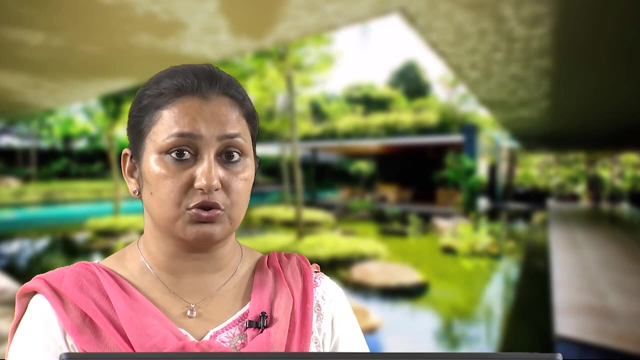 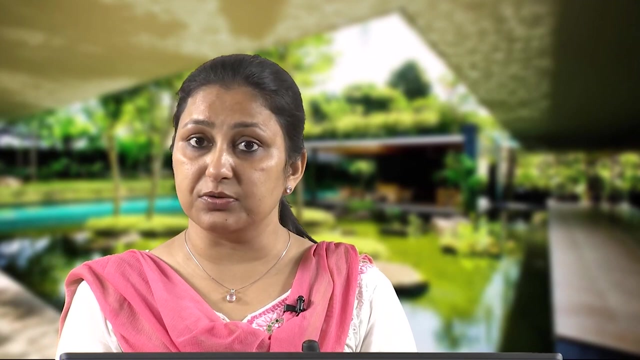 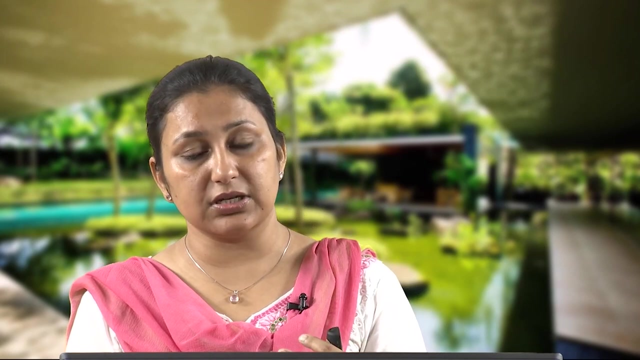 depletion. There were flaws in the kind of research which had happened, because the research was anyways going on. the scientists were not sure. However, the conceptual model of what is causing the ozone depletion was publicized and advertised through politics, through political agenda, so heavily that it actually led to one of 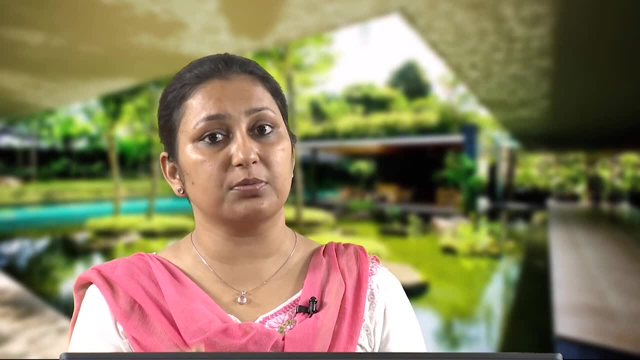 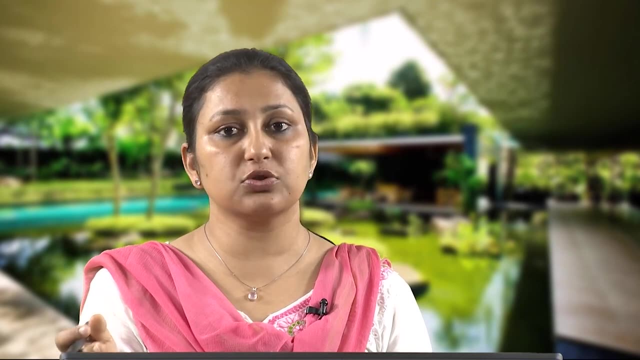 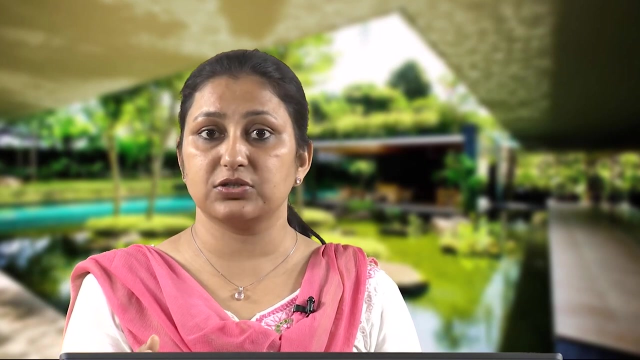 the most successful global treaties, which was Montreal Protocol. In the later years, yes, of course the scientific evidence also pointed to the same fact that, yes, Some compounds, certain elements, were causing the ozone depletion to a larger extent. But at the time when it was proposed as a conceptual model, there was no very strong 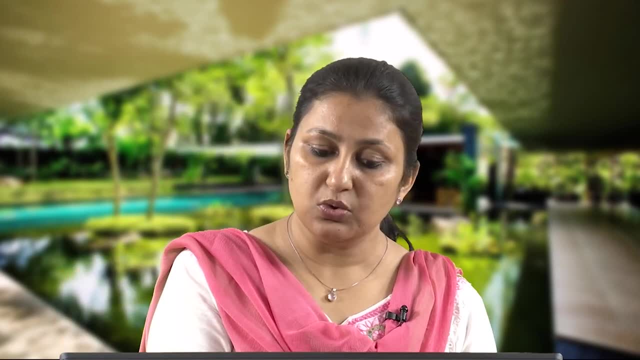 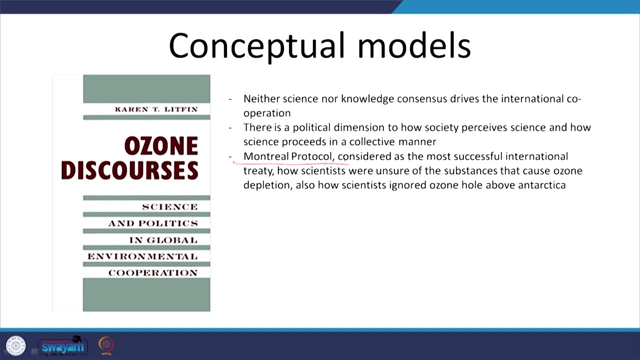 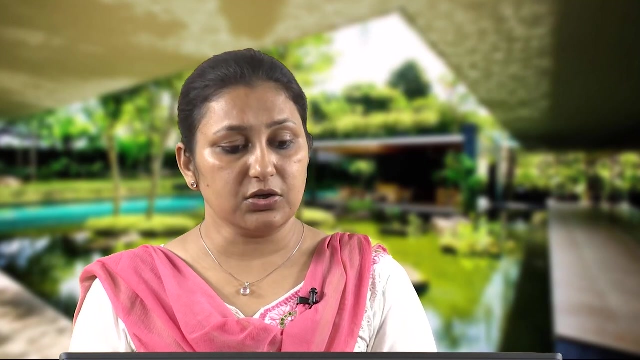 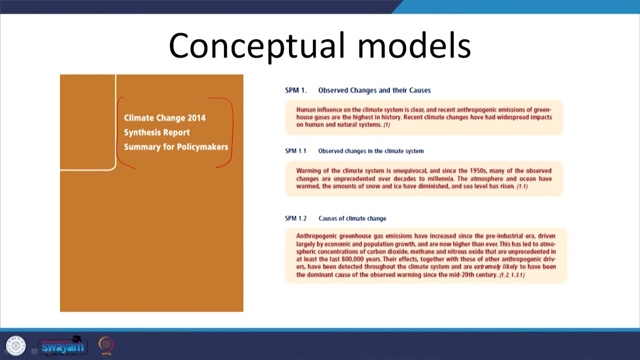 scientific backing. So it actually led to a very successful treaty- Montreal Protocol- which is what usually happens with the conceptual models because they are so heavy on political agenda. It has been good for the world at large. Another conceptual model that we would see Was this, for example, this climate change report 2014.. 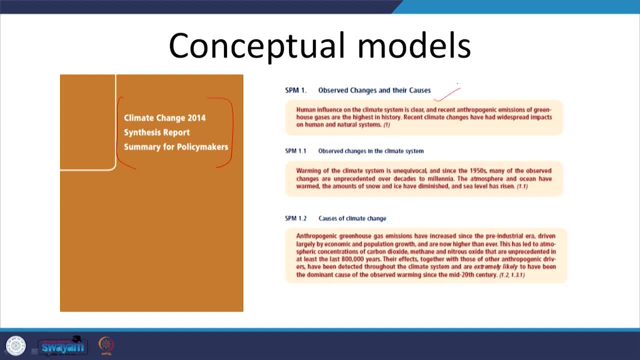 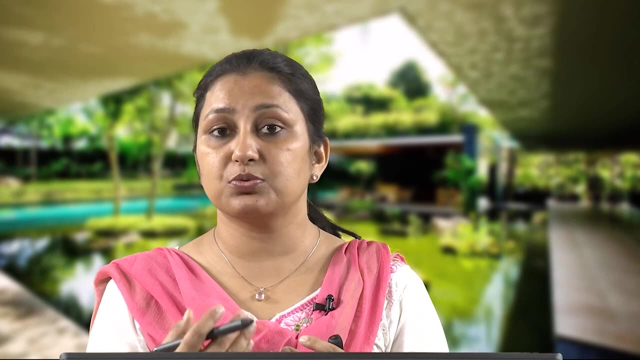 Now it talked about the observed changes and their causes. It observed the changes in the climate system and the causes of the climate change. So, if you remember, there was a lot of uproar on the rate of how glaciers are melting, how it was projected, because there is no scientific backing to it. at what pace will the glaciers? 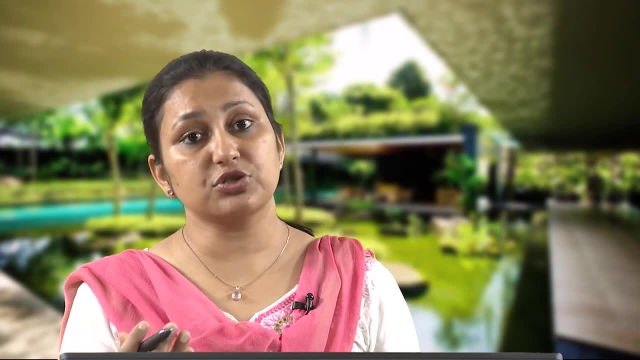 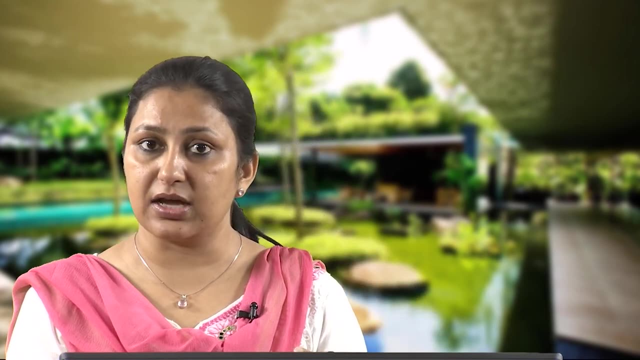 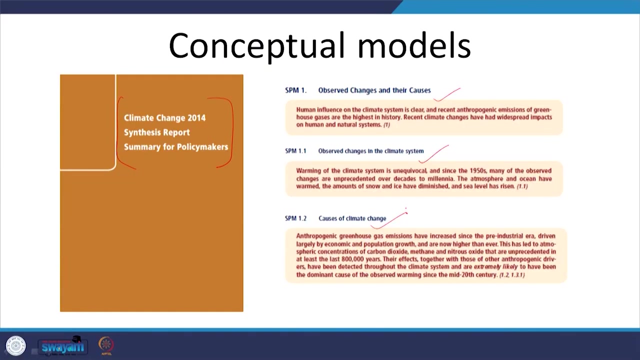 melt. At what rate and in how much time will all the glaciers be melted, and how it would lead to the sea level rise. Yet it brought to the fore the conceptual model that climate change is happening. These are the changes which are happening though, the pace, the rate at which these changes. 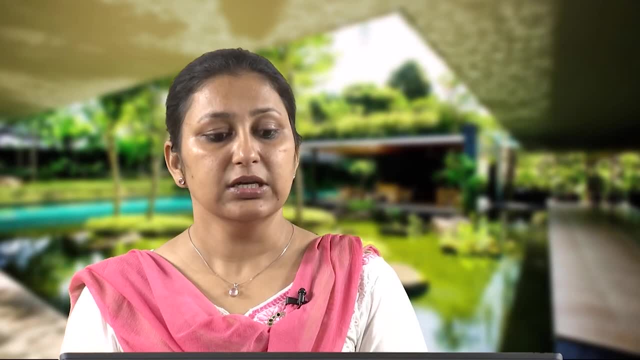 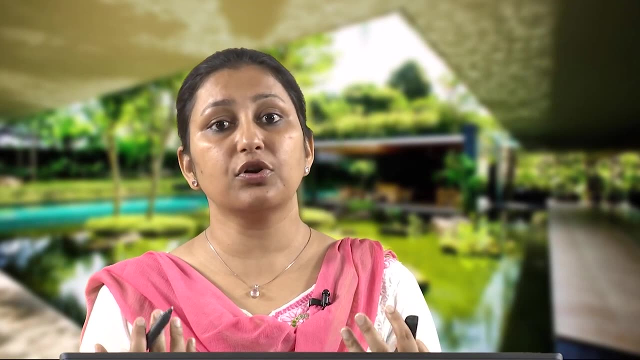 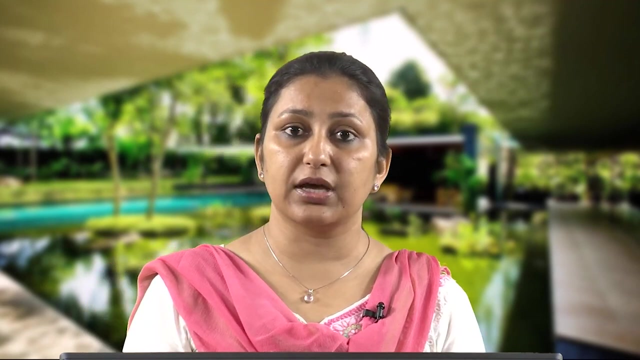 are occurring is not scientifically proven yet, It is good enough. 2. It sensitize people to create an overall large awareness and drive a political agenda where majority of the world comes together to discuss about climate change and to take to act upon it. 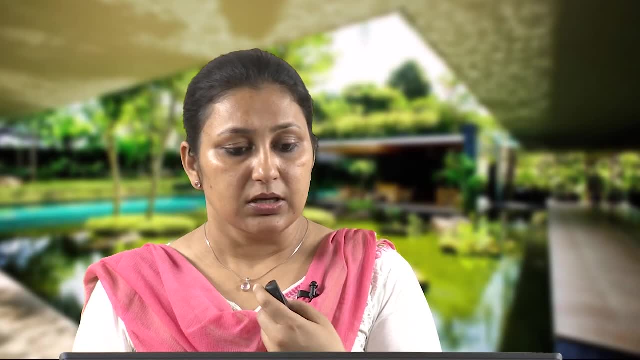 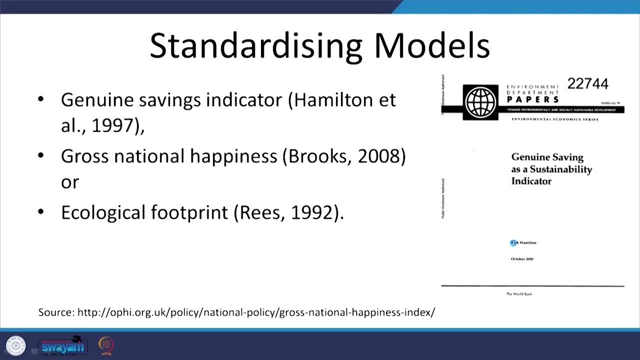 So that is what climate conceptual models do. The last is standardizing models. now these standardizing models develop a new benchmark, a standard 3. 4. Which in reality does not exist. It is a combination of various different parameters put together to lead to a quantity, a standard. 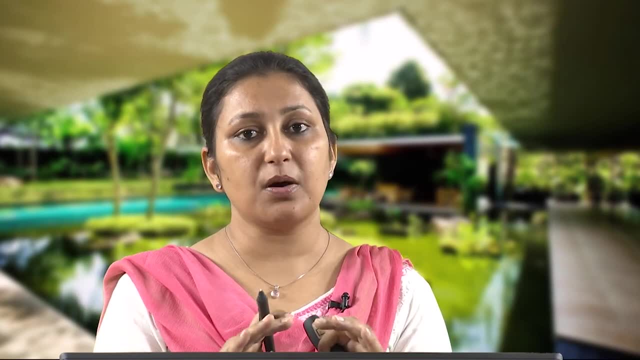 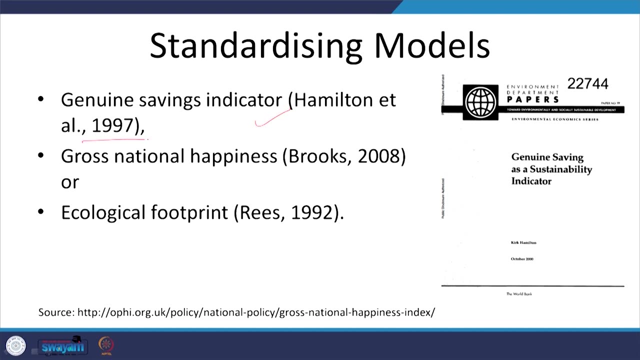 which is proposed and it is counted as a benchmark, For example, genuine savings indicator, which was proposed in 1997, or gross national happiness, which was proposed in 2008.. Now, these are not really tangible, though the parameters which lead to these quantities, 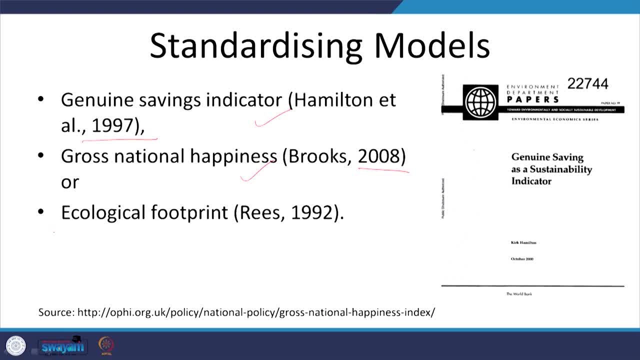 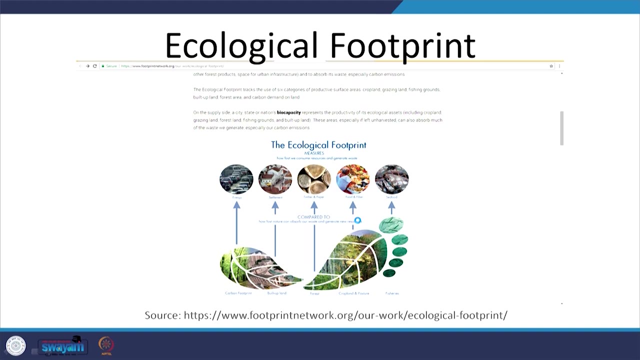 or standards are tangible. Another one which we often see here is ecological footprint. Ecological footprint is a very popularly commonly understood standard, though it in reality does not exist. Let us look at what ecological footprint is 4. So ecological footprint actually measures the amount of resources which we consume. 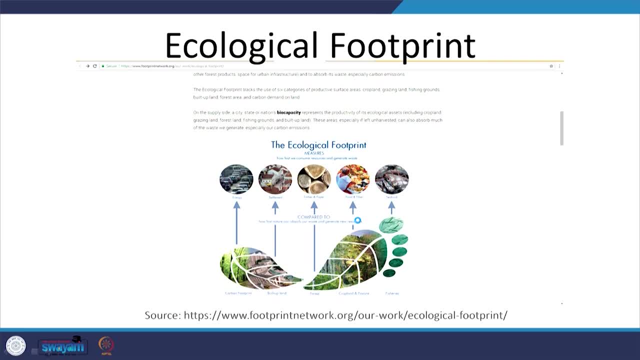 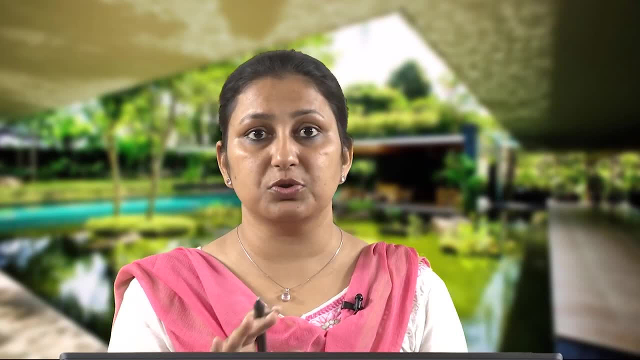 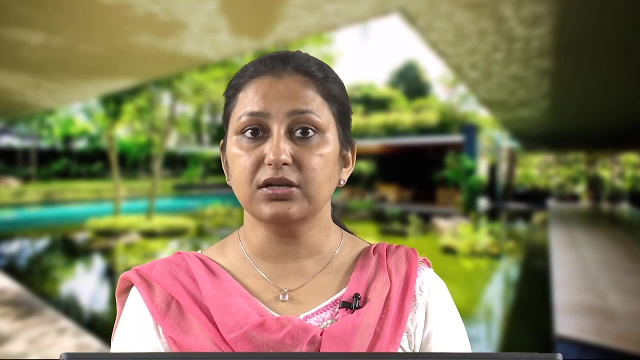 It could be per capita basis, it could be per state or nation or for the entire World. how much of these resources are consumed per capita is what our ecological footprint is, and how much of ecosystem, land, water, trees, plants, agricultural area, farm land is required. 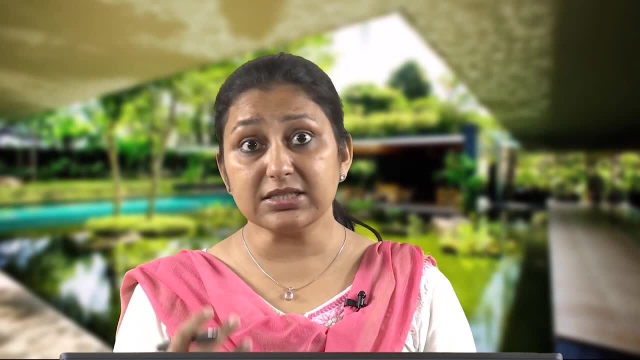 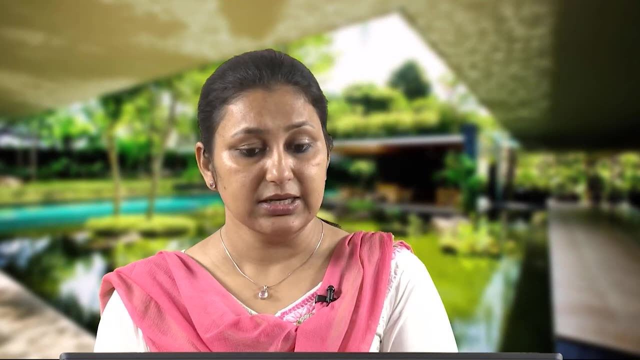 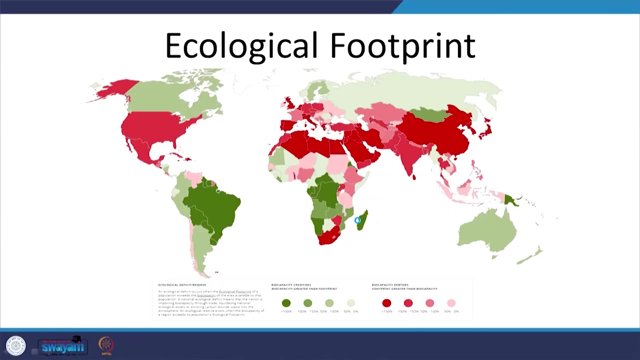 to rubber, for example. 5. is required to sustain the kind of lifestyle which is being discussed, for which ecological footprint is calculated. So there are websites which are available. you would see a link of these websites and you can actually go and visit these websites where the ecological footprint 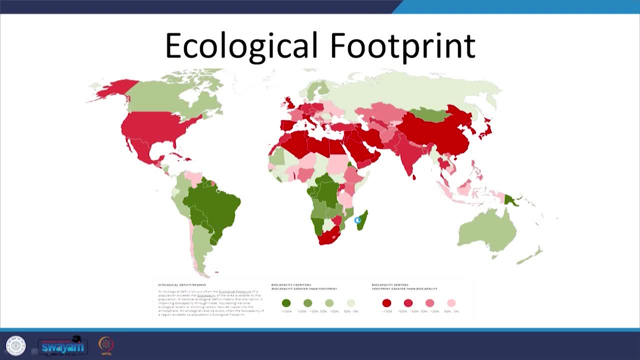 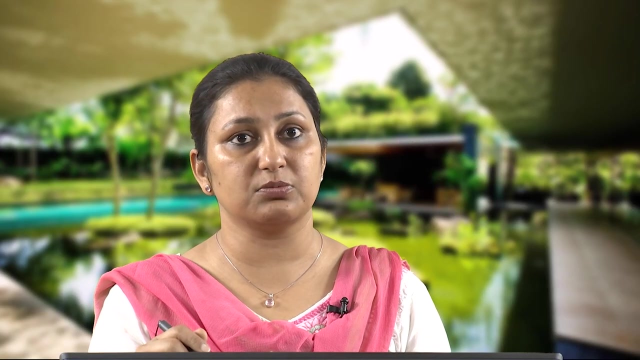 of the entire world. different nations has been calculated. Now the ones that we actually see in reds have a larger ecological footprint than the amount of resources which are contained within the boundaries of these countries. A darker of red implies that the resource consumption, the rate of resource consumption, is much higher than the amount of resources which are available. 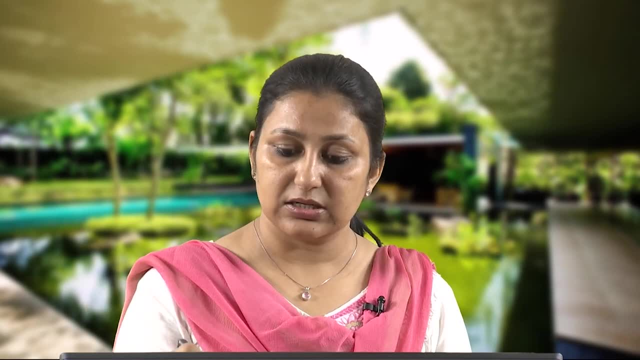 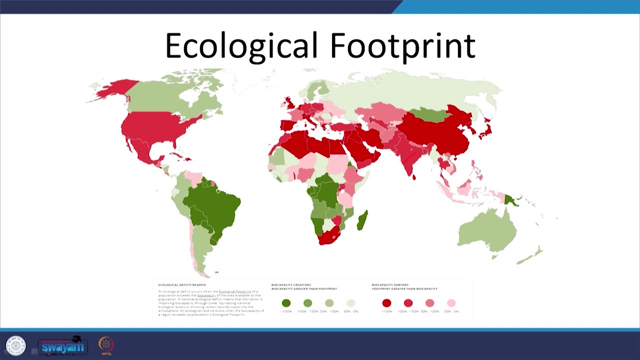 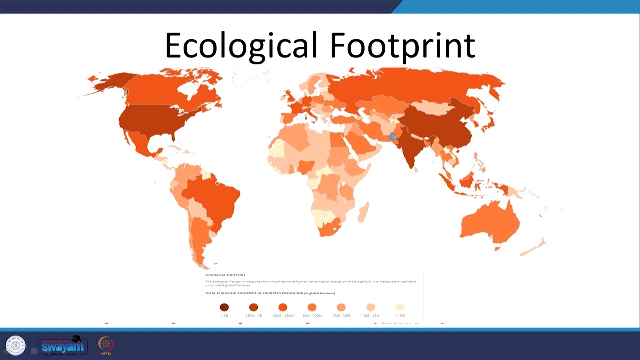 within their boundaries. So we can see that India, our country, is quite intensely using the resources. We will see whether it is per capita consumption of resources or it is the consumption of resources for a nation at large. So this is looking at the ecological footprint of on the basis of country's population. 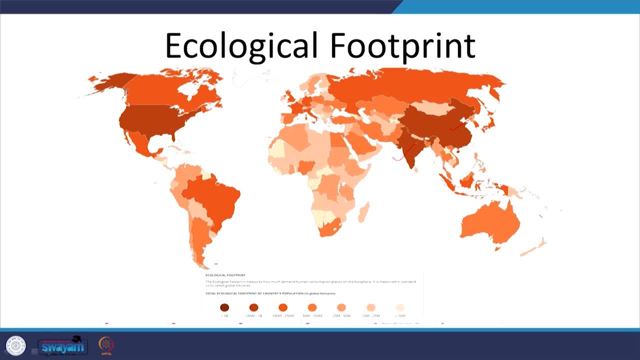 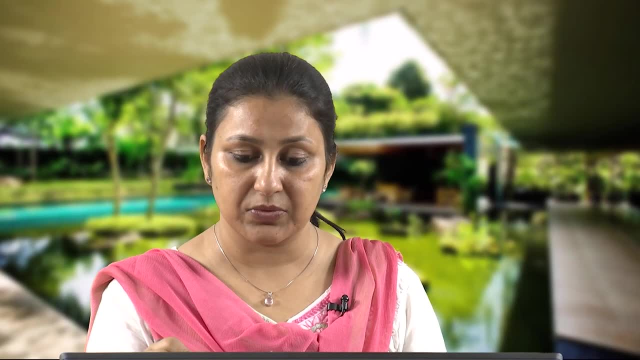 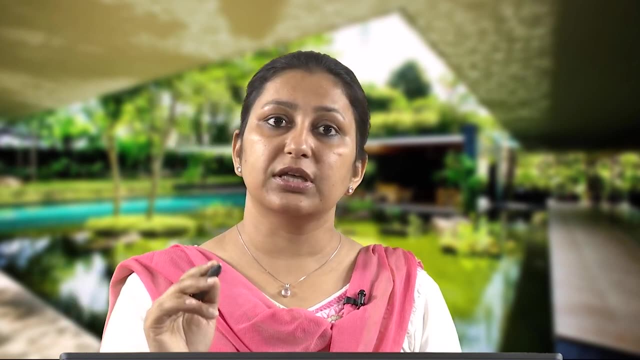 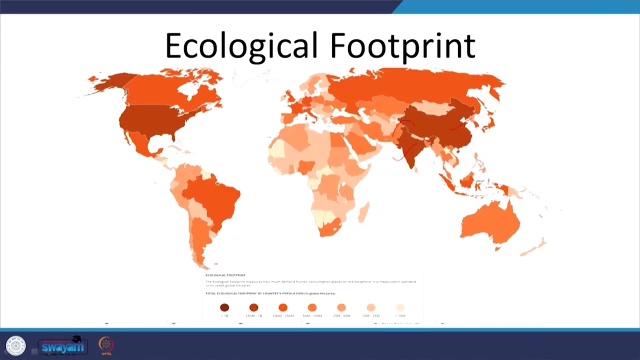 The darker of the red implies there is a higher concentration of population, and that is why the ecological footprint is much higher than the amount of resources which are contained within the boundaries of these countries, Countries which are sparse, where population is less, even though their per capita ecological footprint may be higher overall for the country. 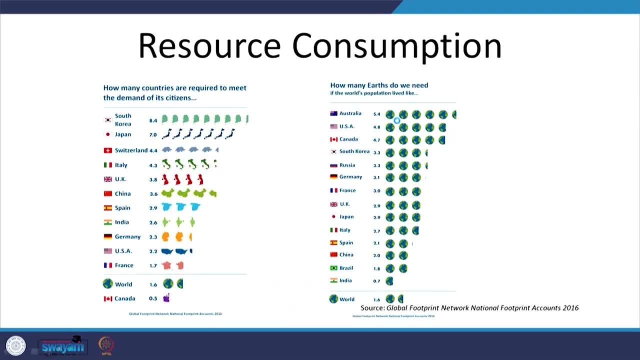 they will still have a smaller ecological footprint. Let us look at this resource consumption chart Now. here we see that, given the kind of lifestyle people in a country follow and the way they consume resources, how many countries of the same size are required to meet the demand of its citizen? So this is resource consumption. 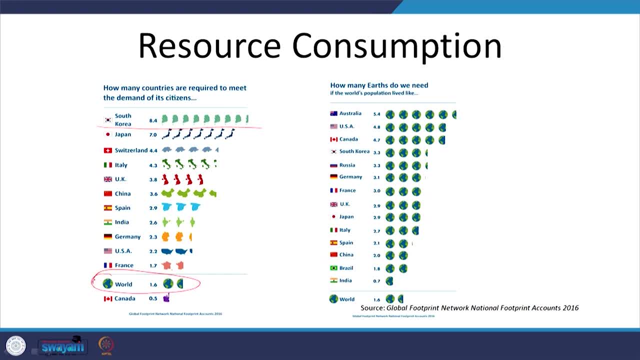 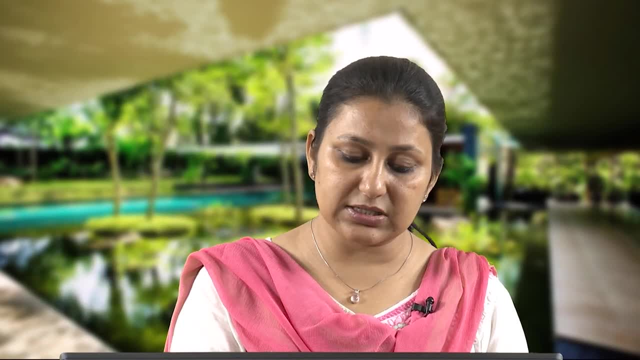 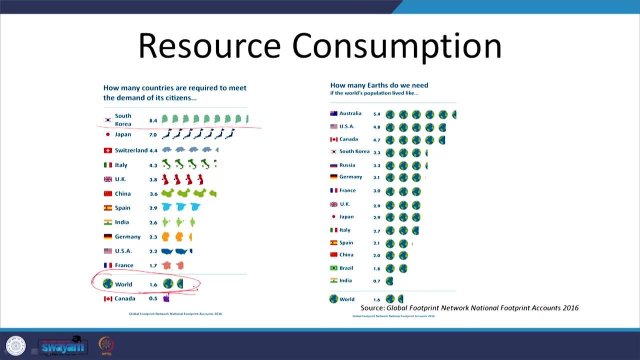 If we look at the world here, the rate at which the global population, the world is consuming resources is we would need 1.6 times the earth to fulfil our demands, fulfil our needs for the resources. We can also look at this very interesting piece of information: where if the world's population lived? 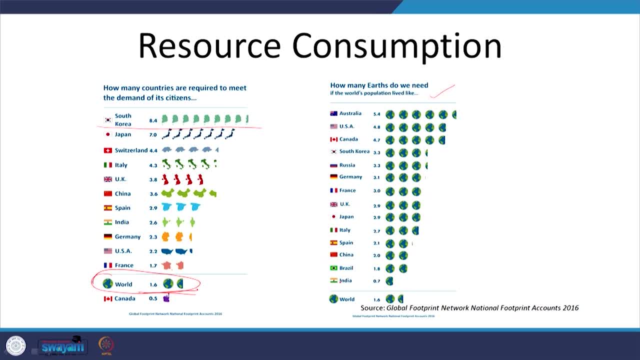 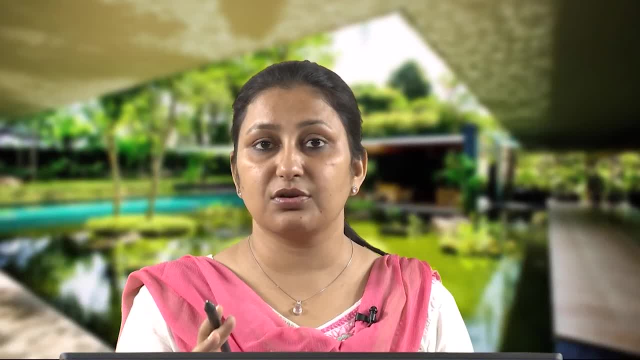 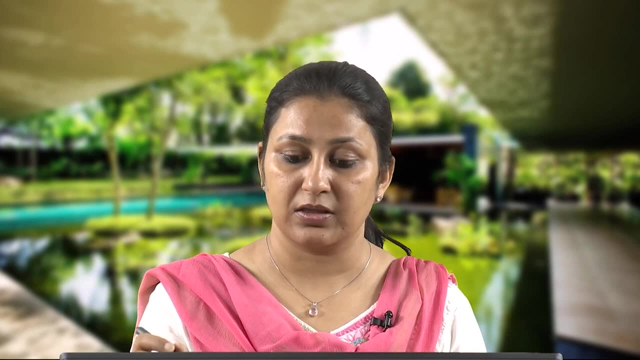 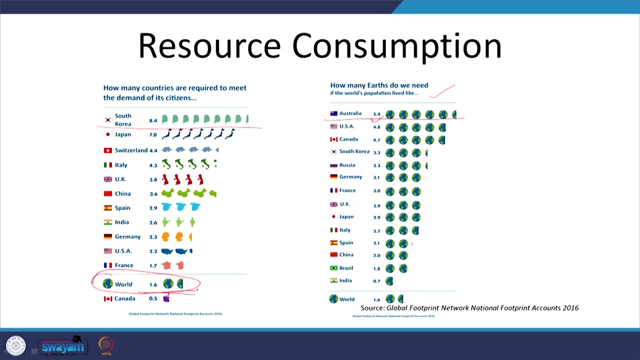 like the population in these countries, the way people are living in these countries. how many earths would we need like that? So it is a direct representation of how sustainably people in different countries are living the lifestyle which we say. So if people live like the way Australians do, we would probably require 5.4 earths to fulfil our 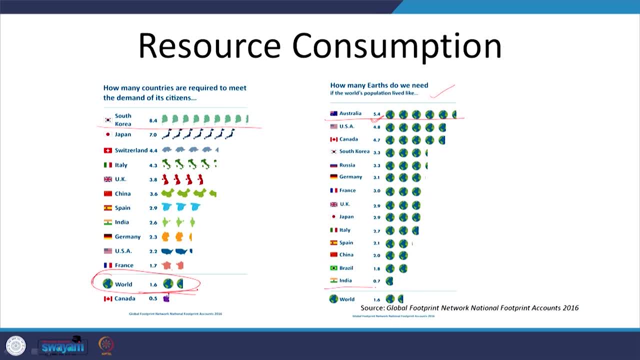 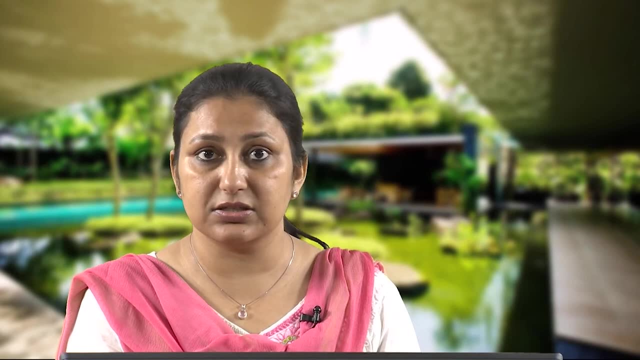 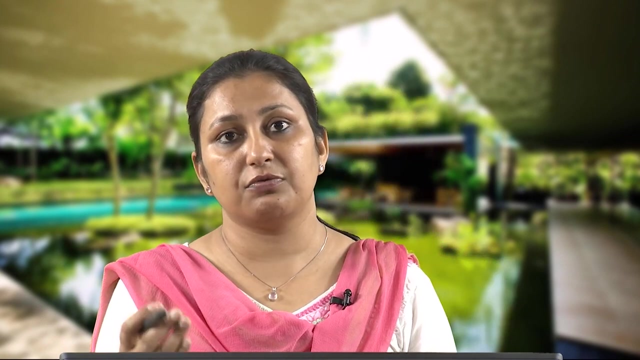 needs. However, if the world lived like the way Indians live, even today, we would need only 0.7 of the earth. earth, that is, if the entire world starts living like the Indians do. However, there are a lot of associated facts and issues which need to be discussed. 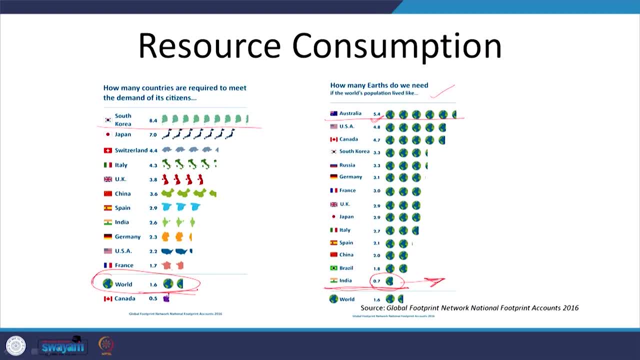 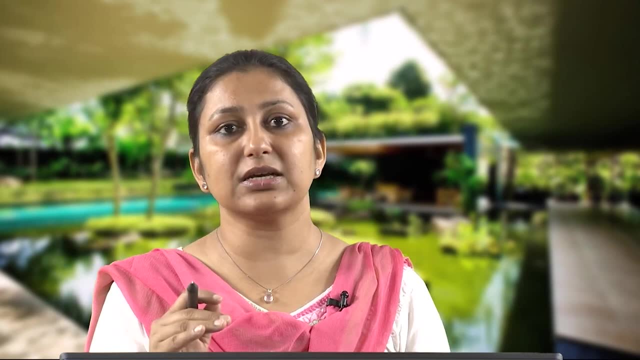 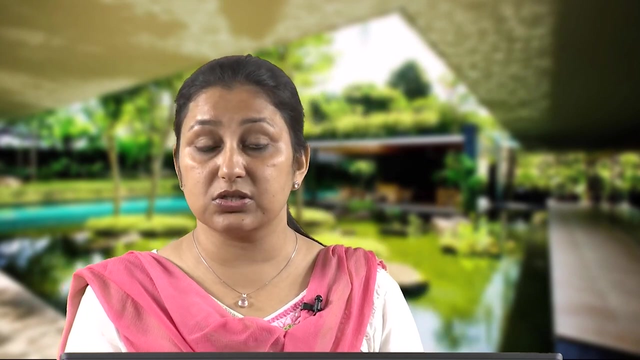 We must very clearly know when I am saying that if the way Indian population lives, we are also talking about crores of people who are living below the poverty line, where they do not have access to the basic amenities of life. That is why, probably, per capita resource consumption is quite low for a country like ours. 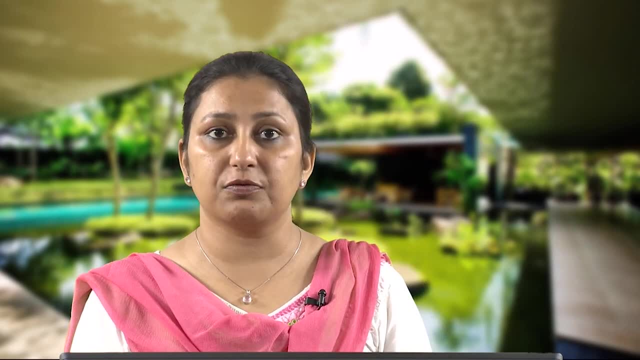 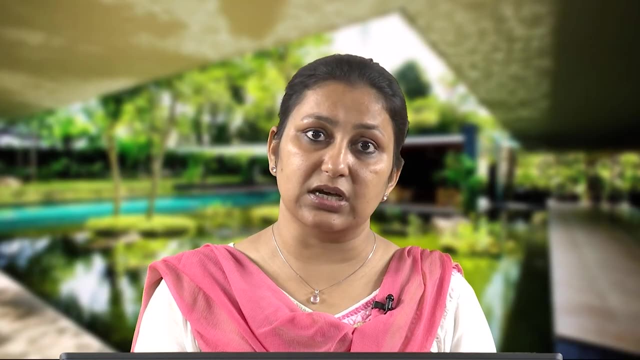 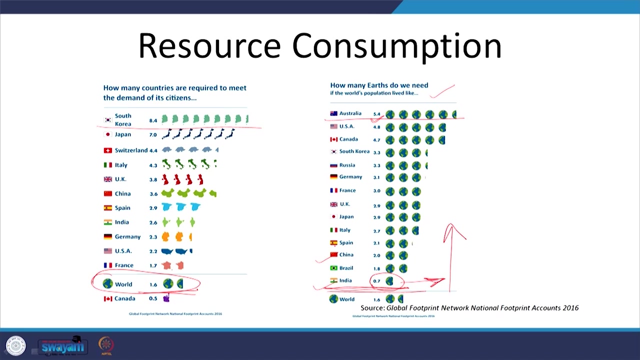 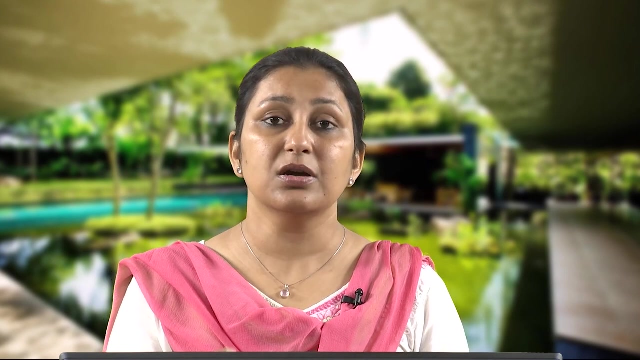 And as we go on with improving the quality of life, this resource consumption is bound to increase. We will not be able to survive. We will not be able to sustain ourselves and also, given that countries like India and China have very large concentration of population, the per capita increase in resource consumption. 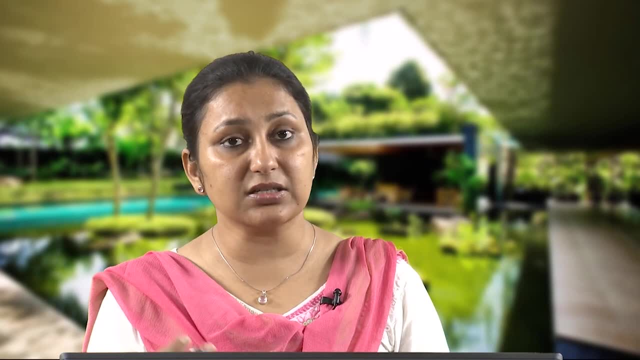 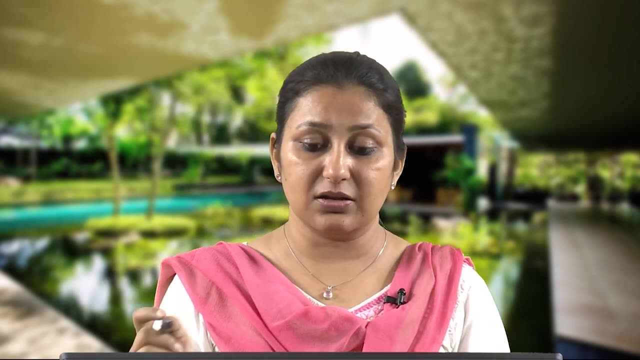 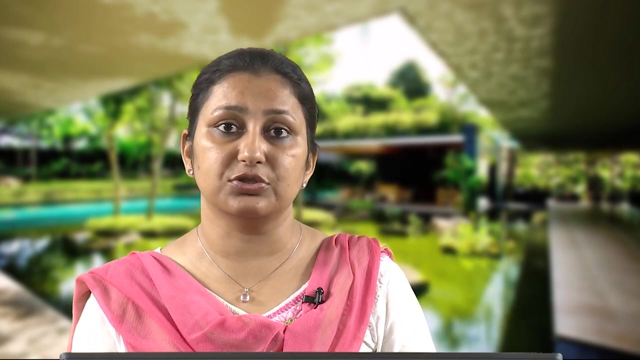 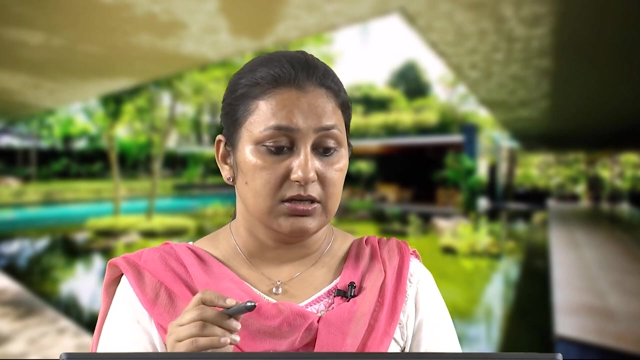 multiplies with the population and suddenly makes a bigger number. So this is a very interesting fact to see, and while I was saying that, if we continue to live the way we are living The world at large, we need 1.6 earths to fulfill our demand. 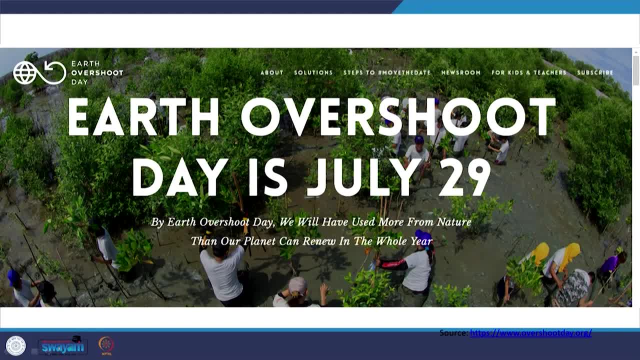 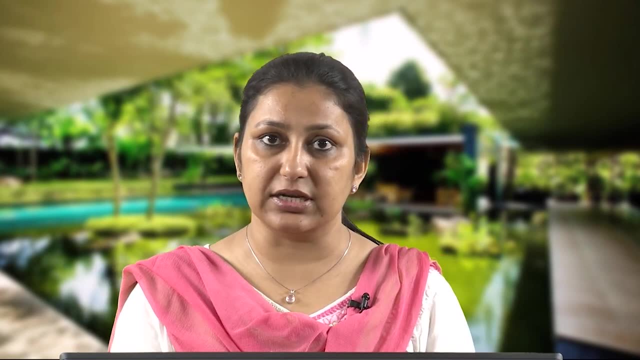 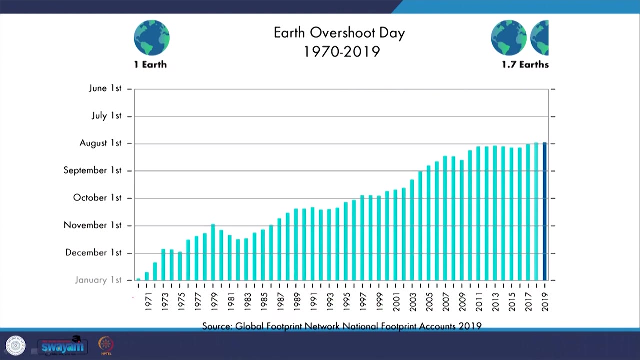 So, looking at that, there is a concept of earth overshoot day, where the resources which are available to us for an year have been already consumed by a particular date. So this has been coming down. If we look at the historical data, we would see that around 1970s we were almost consuming. 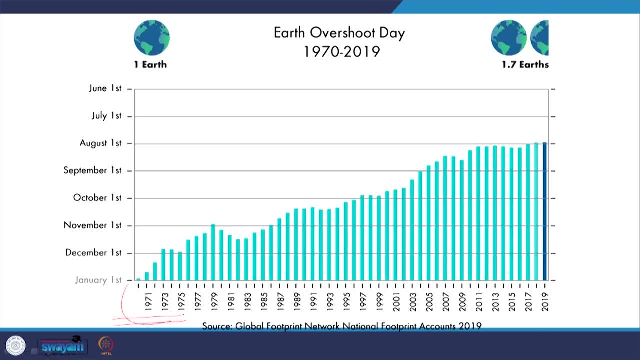 the amount of resources which were available for an year, in an year only. However, when we are coming to 2019, we are exhausting the resources by July 29th. So we are short of resources. We are short of this much period. 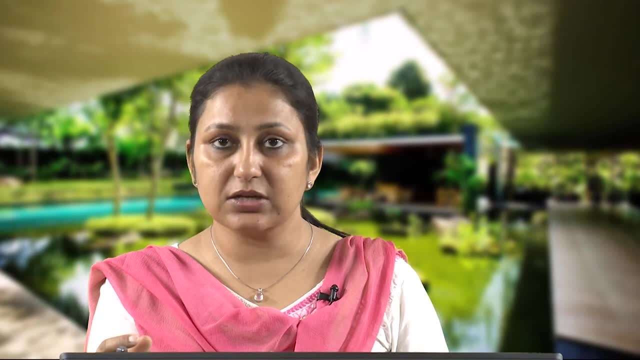 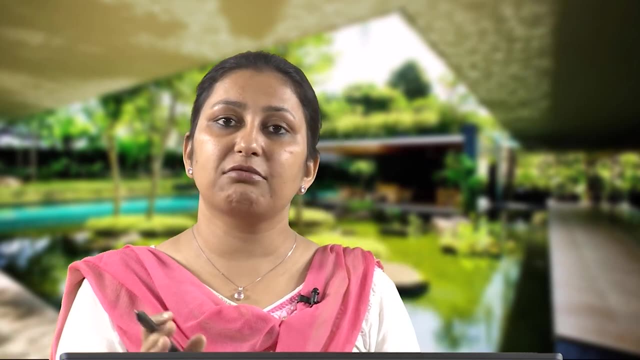 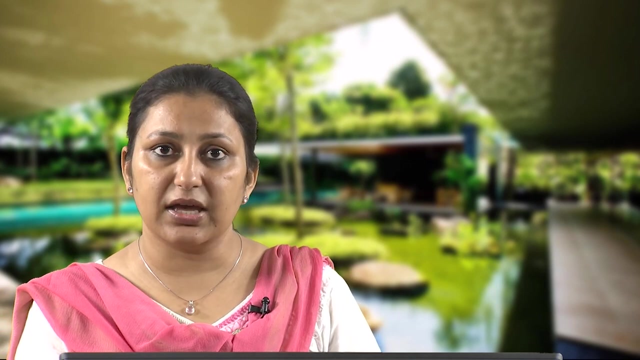 Now, if we total it up, so every year we are reducing it by, say, 5 months. we are reducing it by 5 months in one year, and like that, we have very little time left on earth to survive. This is the reason why all of us must act now, and specially we are talking about country. 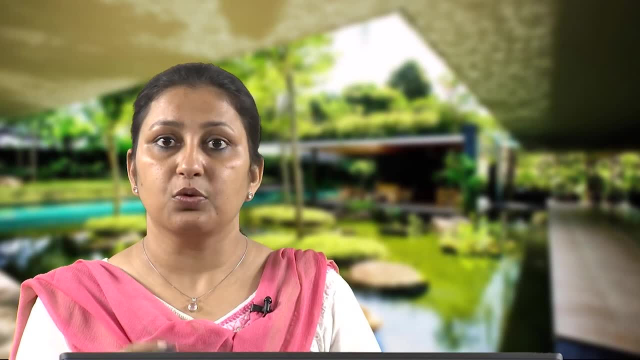 like ours, India, which is a developing nation, We yet need to provide the resources which are available to us. So this is the reason why all of us must act now, and specially we are talking about country like ours, India, which is a developing nation. 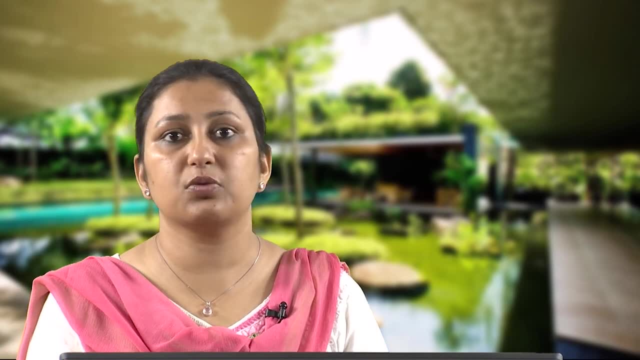 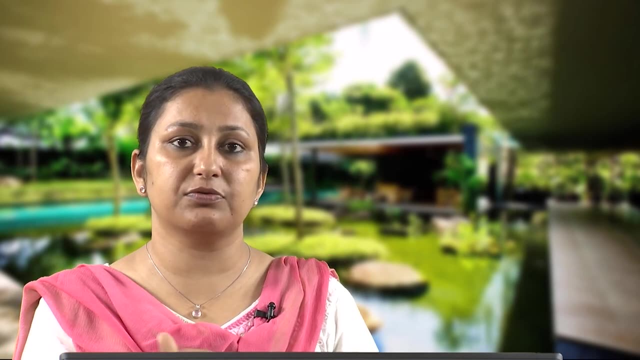 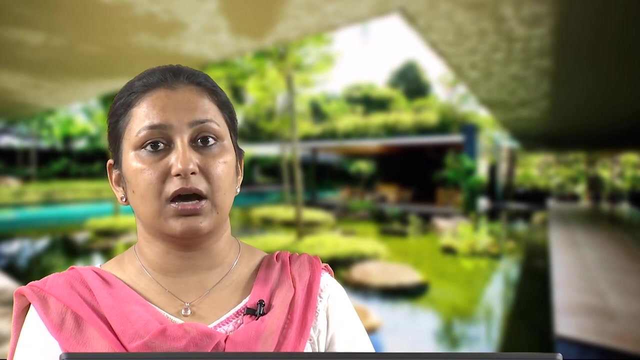 We yet need to provide the basic facilities to our people of drinking water, of shelter. If we do not move ahead in a sustainable manner, it will be very difficult for us to sustain the growth, sustain the population in a healthy manner and provide the same amenities. provide. 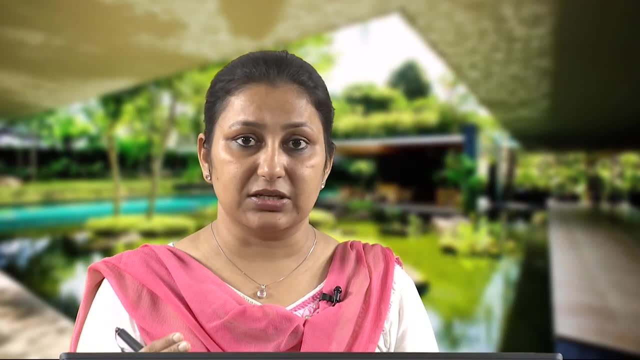 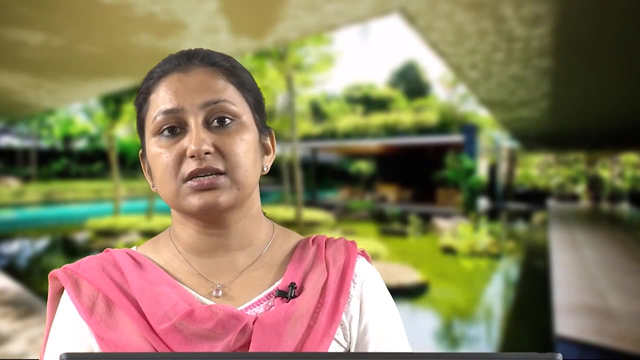 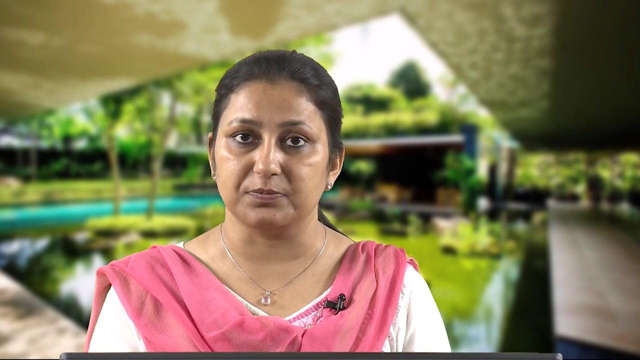 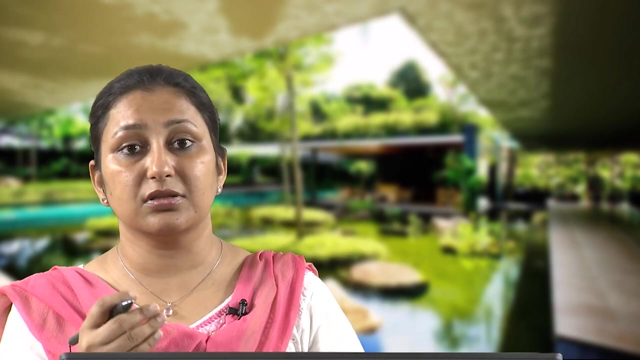 the same quality of life to our future generations. So with this I will close this lecture 3, where we will discuss about the importance of sustainability, where we have discussed what are the different concepts, different definitions through which we can understand sustainability. As we move on, we will discuss how sustainability has come to the point, the way we are discussing. 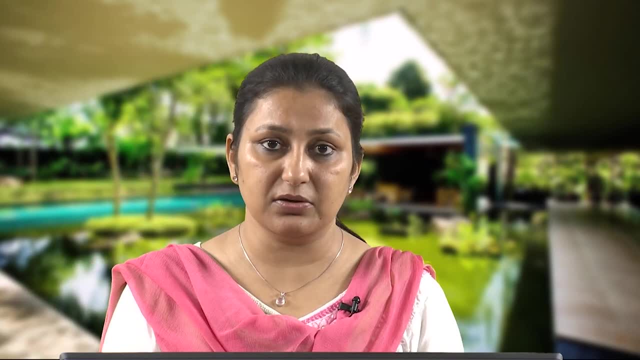 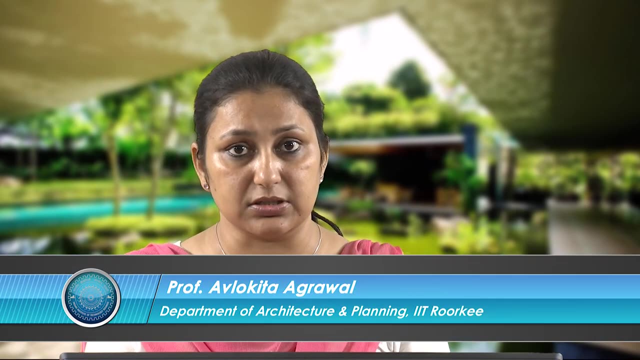 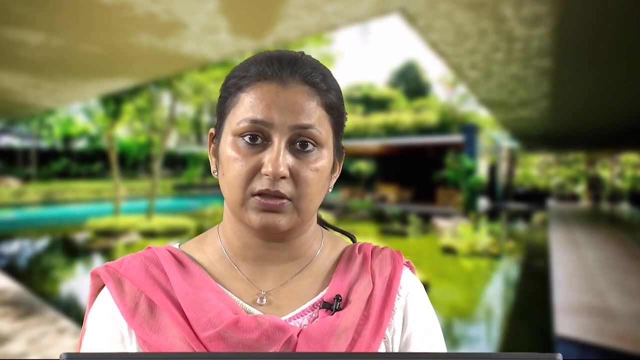 today. Has it always been discussed in the same manner like we are discussing today, or were there different issues which people talked about when they were talking about sustainability previously, Say couple of decades back, or almost a century back, or more than that. So see you in the next lecture. goodbye. Thank you.